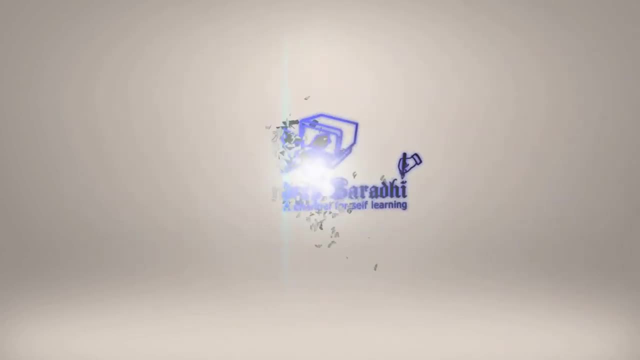 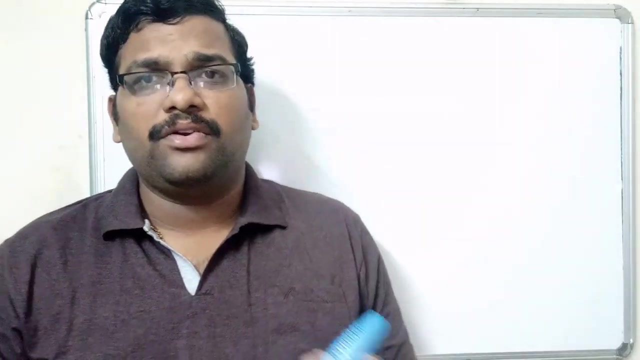 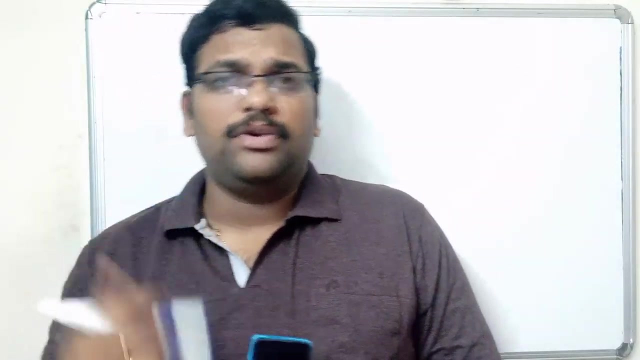 Hello friends, welcome back to our channel. So in the previous session we have seen the object-oriented concepts introduction in Python programming. So whatever the language it may be, the concept is same. So object-oriented concept. So we have seen all the introductions about this. 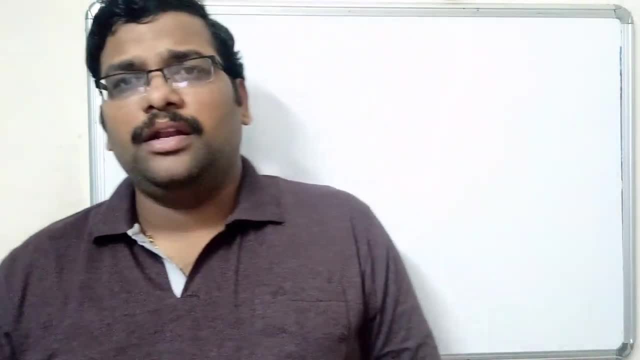 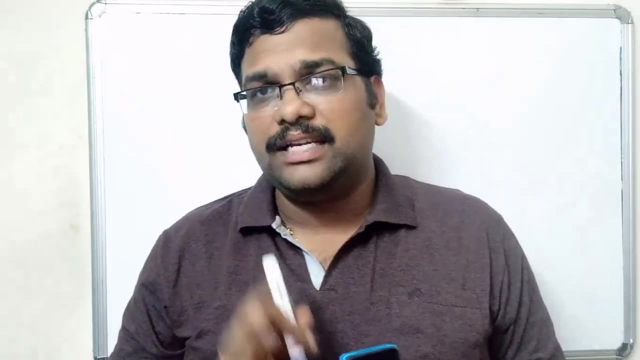 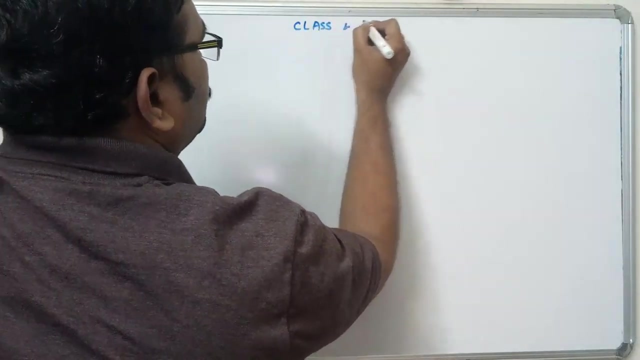 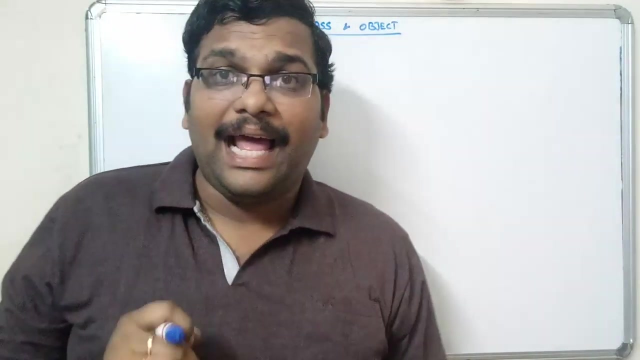 class, object, abstraction, encapsulation and inheritance and polymorphism. So in today's session we'll go with the class and object, So how to create a class and how to create an object Right, So a class can be having both the attributes and the behavior. 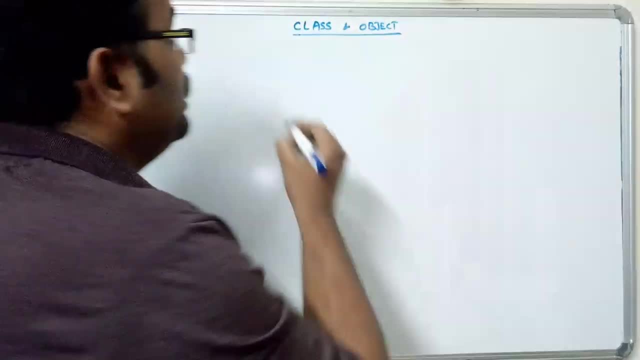 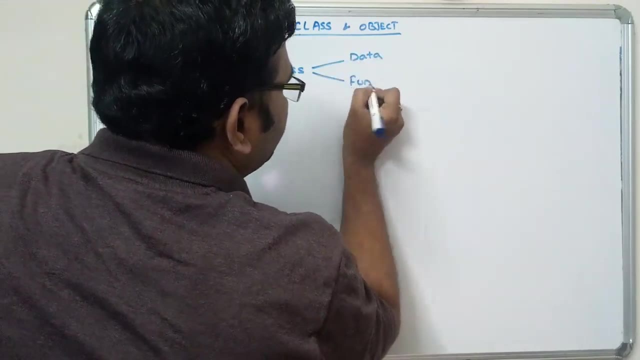 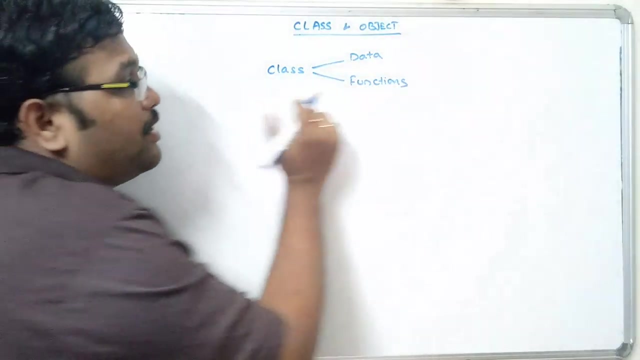 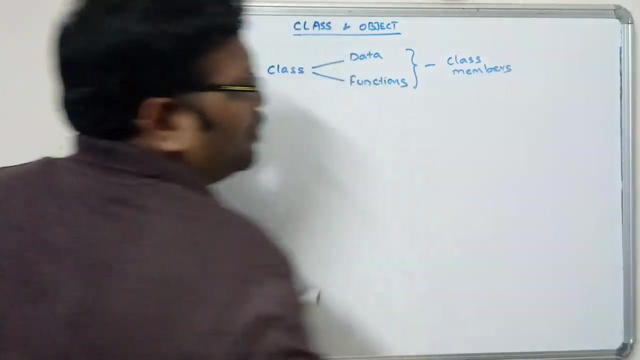 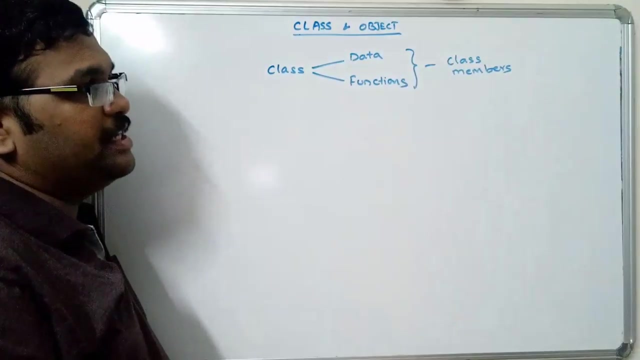 So that we call it as data and functions. So class can have the data and functions, So both the data and functions will be combined and called as a class And these two are called as class members. right, so how to access these class members? how to access these class members? that means either data. 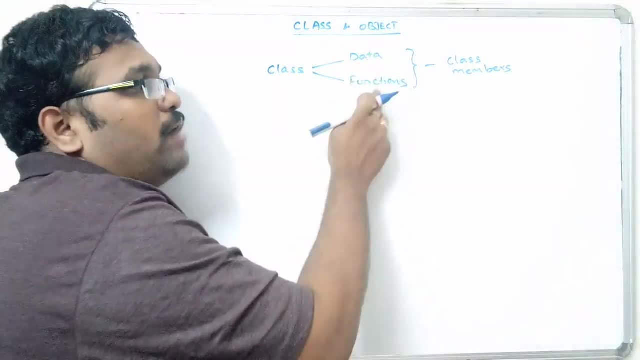 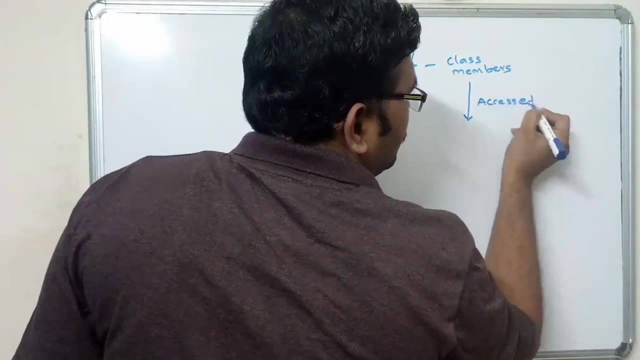 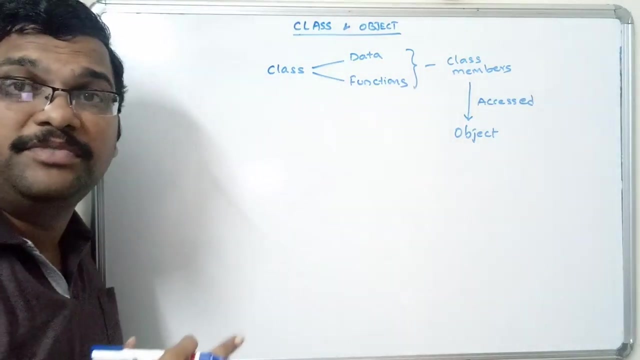 or functions. so how to access the data or how to access the functions of a class, so that can be done, accessed with the help of object, with the help of object. so if you create an object, with the help of that object we can access the data and functions of the particular class. so this: 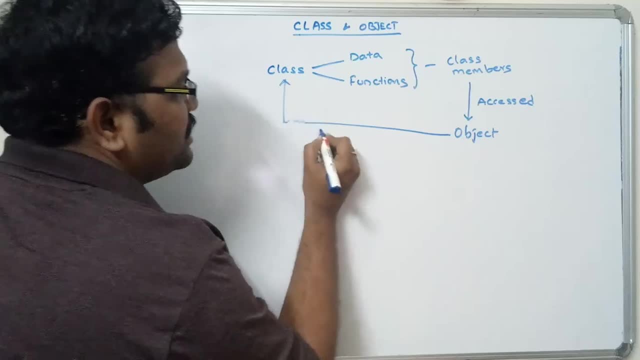 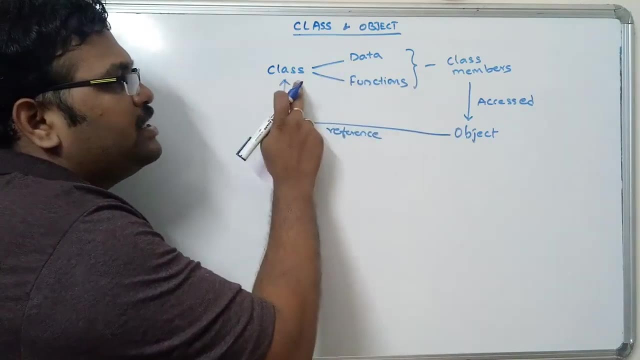 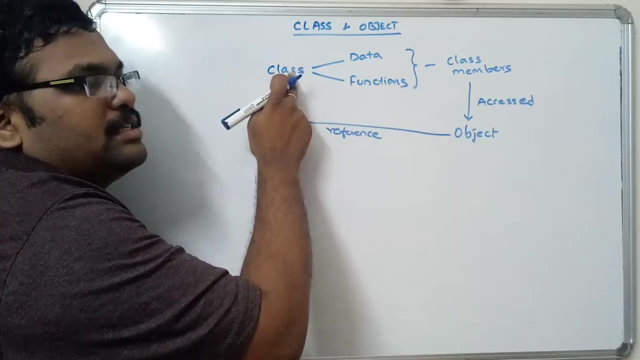 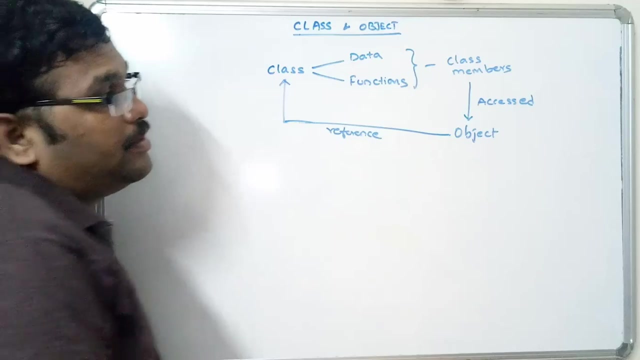 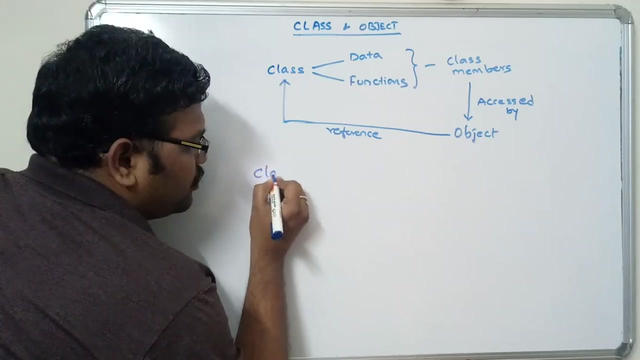 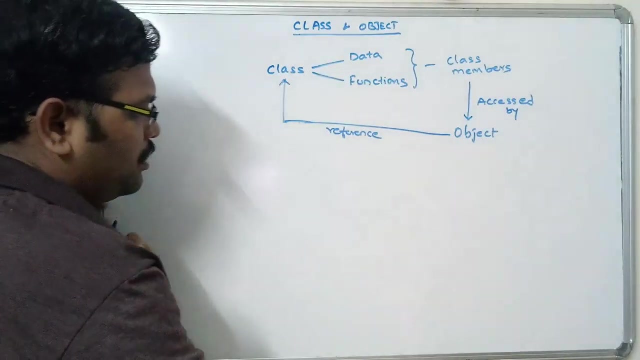 object is a reference to this class, reference to this class. so once a class is defined with the data and functions, an object is created as a reference to the class. so that object, with the help of this object, we can access the class members right access it by an object. so let us define here. so let it be class having sorry, so let us. 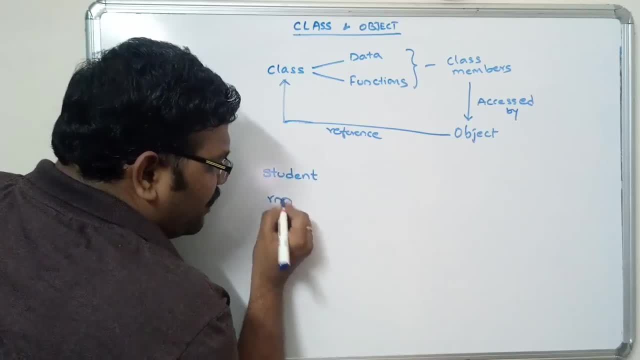 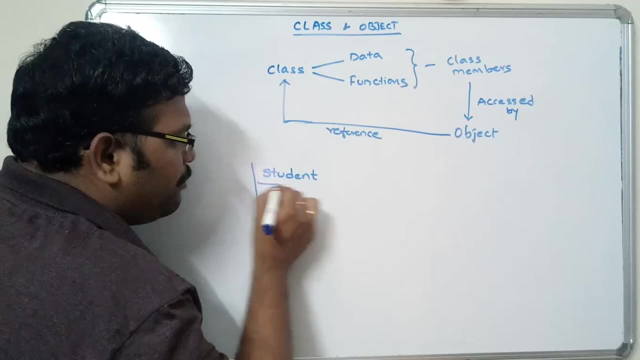 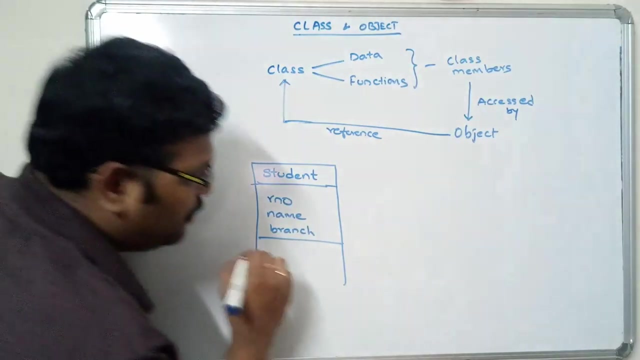 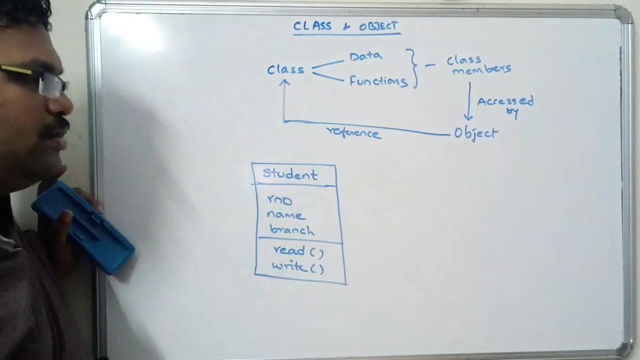 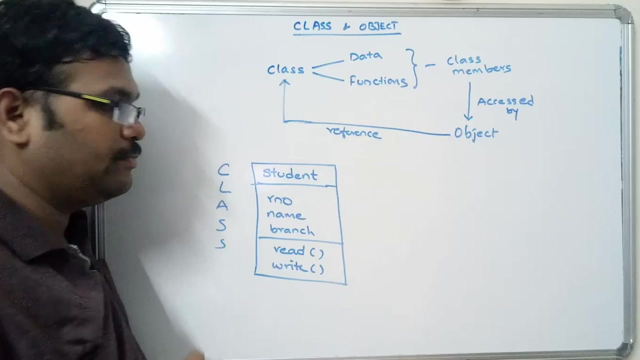 take a student as a class. a student class is having our number, name and a branch, so three attributes, or simply we can call them as three variables, or the data. okay, the data and functions. we can use a read function and the right function, right? so this is called a class and for this, in order to access this one, we have 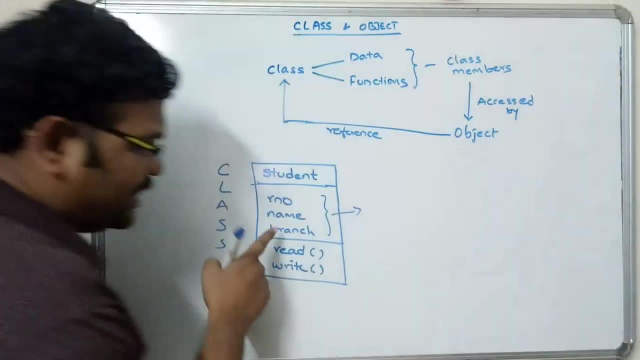 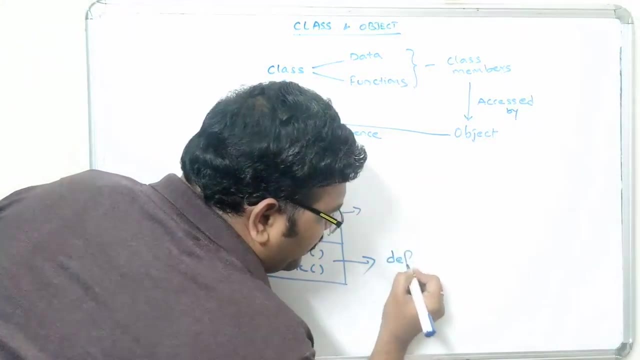 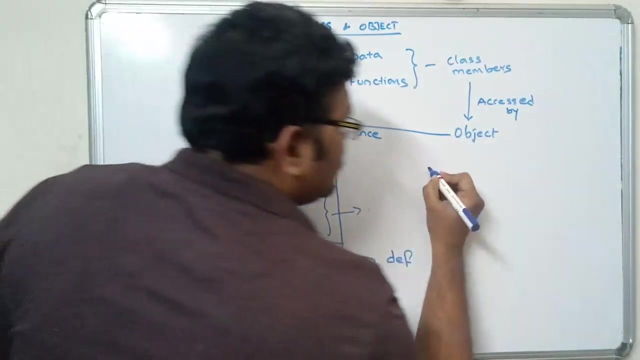 to create an object. so how to create a. so these are the data and these are the functions. we know the functions always starts with the DEF keyword. the same way here we will write. so a class can be represented in Python as a class, so it should be. the class should be defined by using the class. 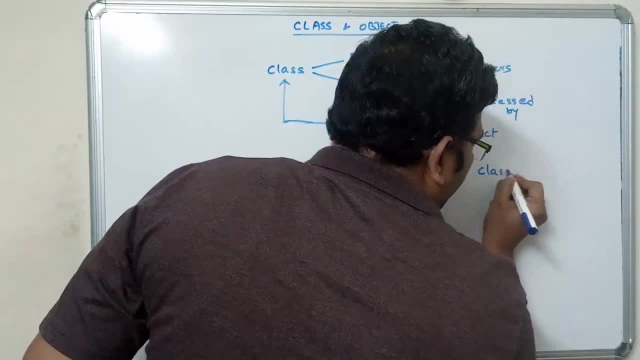 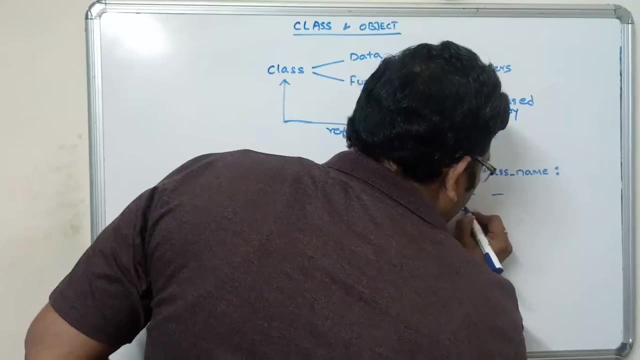 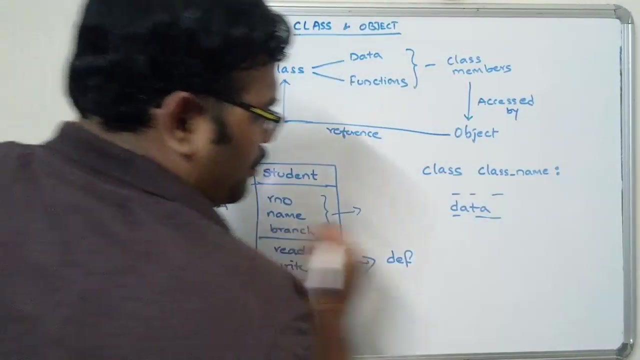 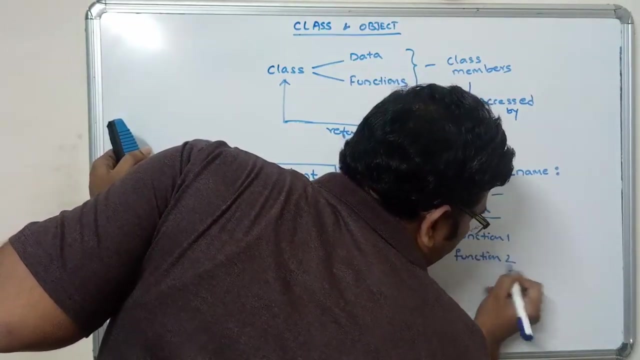 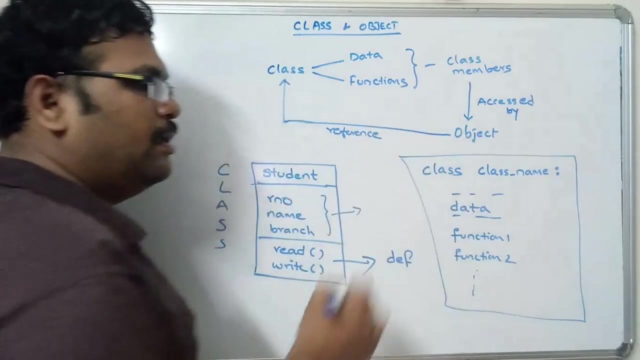 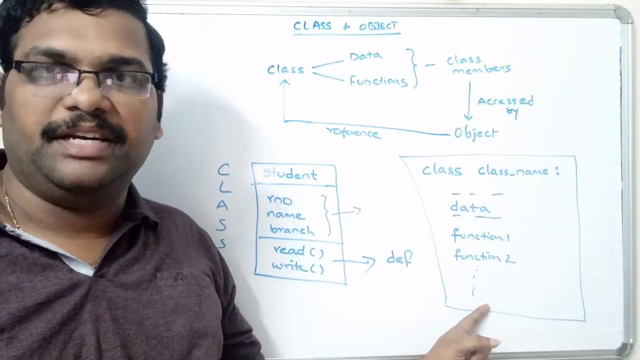 keyword, so class, followed by the class name. it's a block of statement. so this is the data and the shows and functions: function one, function two and so on. so this is how we can represent a class in Python. so here in Python programming, a class is a block of statement, class represents a block. 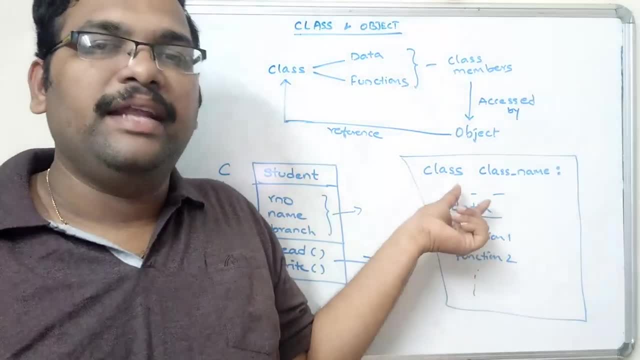 of statement. so here we should write both the data and the answer to which class is, which is objective. so it is very important to learn classes now. we already know that, that which will form the data and société, because the class will be derived from the data and the answer to which class is derived from the data. 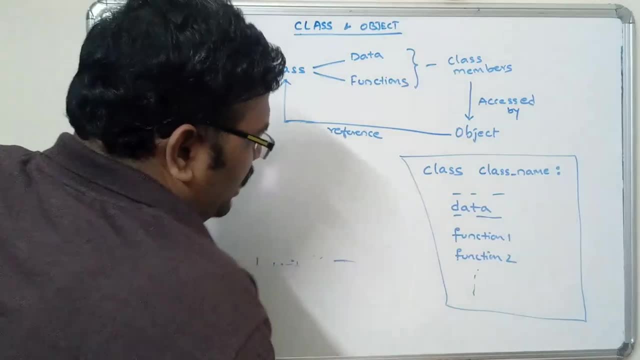 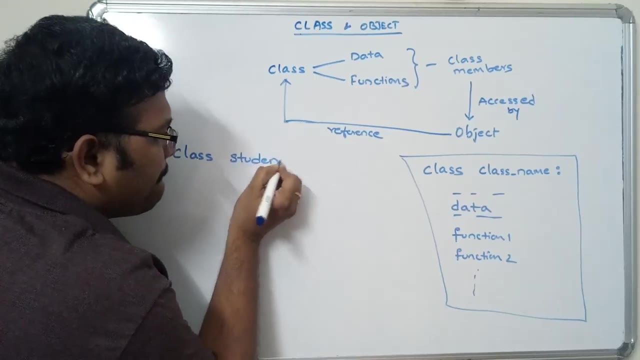 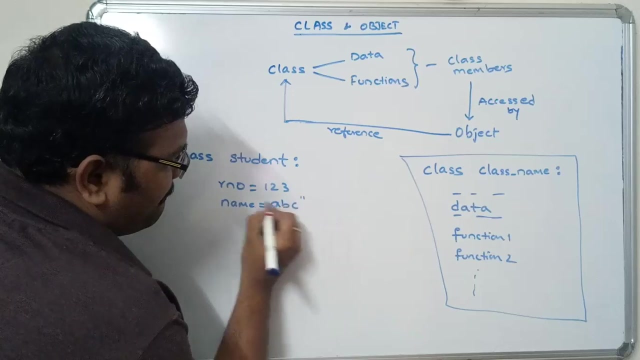 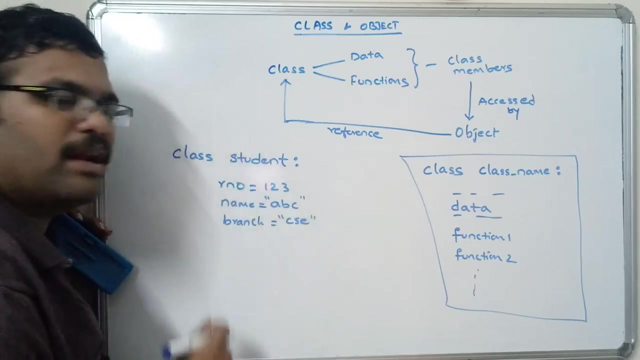 and functions right. see, I will write a students class, so class. student, block of statement, so indentation. then here we can write the data: R number is equal to some 1, 2, 3, some name is equal to some ADC, some branch is equal to CSC. so whatever the data we can 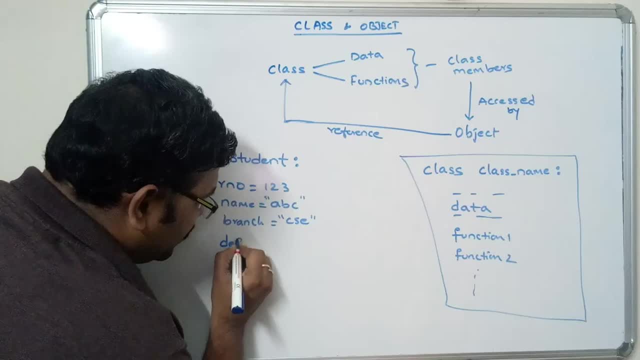 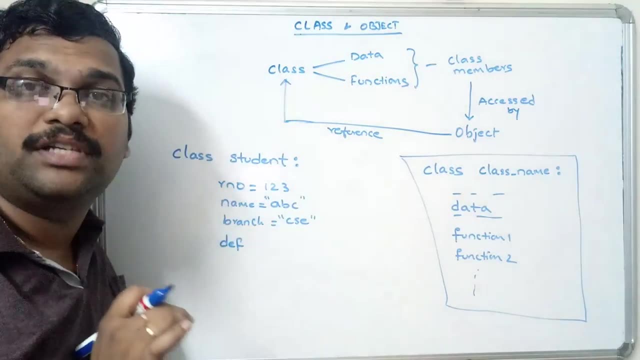 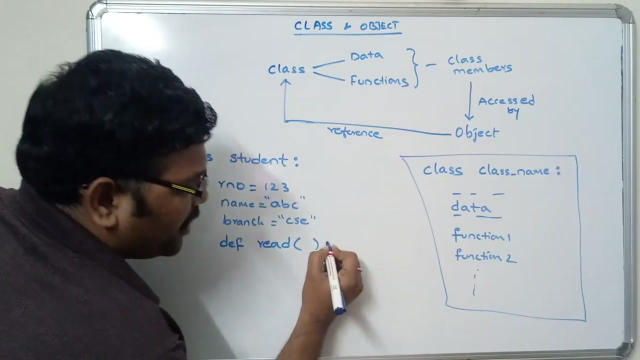 write here so, and then functions. so we know that the functions it say use the different functions, but these are implemented in a class, so every function should start with the D E F keyboard. so D E, F the function name. so read colon. and because it's a block, you're just, I'm writing only the print statement, so I'm. 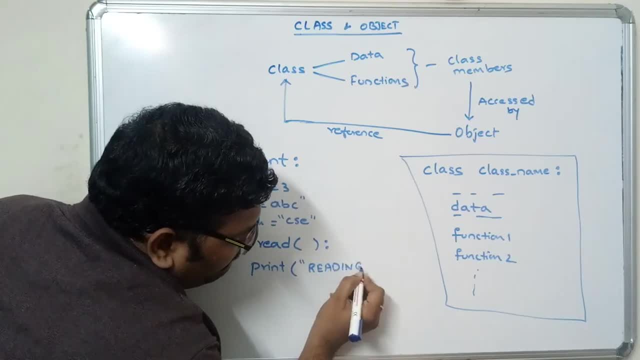 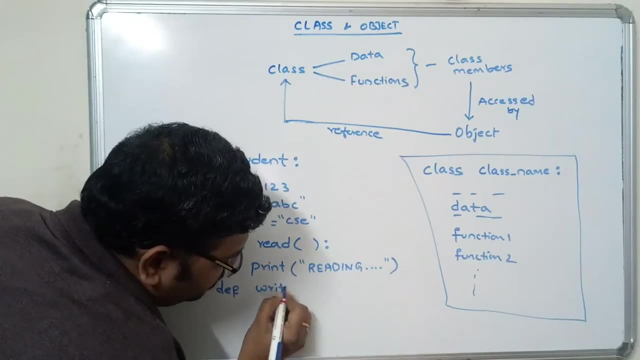 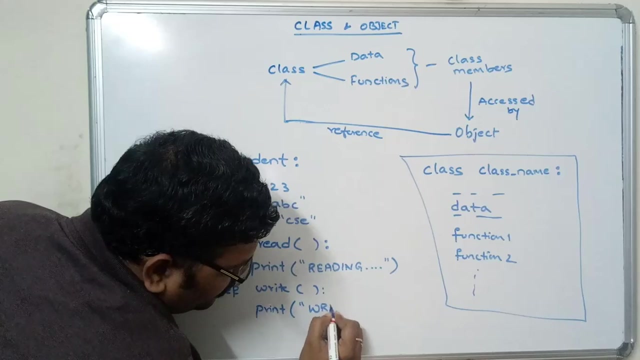 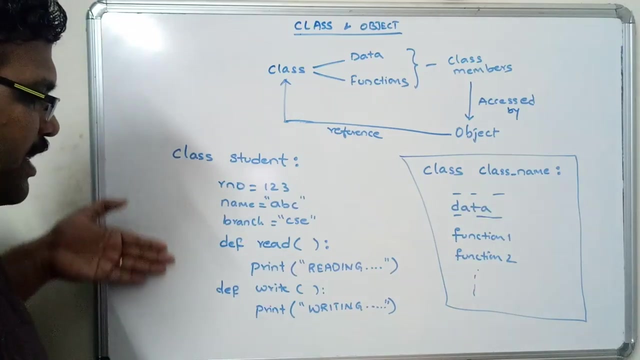 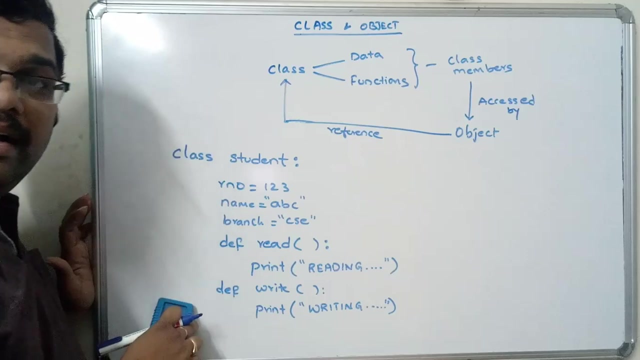 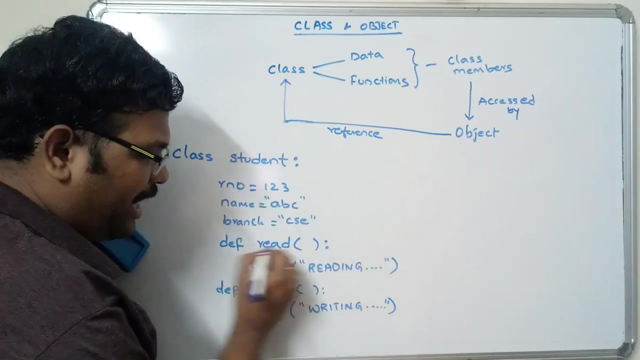 writing only the print statement. so reading similarly: D, E, F, write, function, print writing. so this is how we can create a class. so outside the class, that means after ending the block of statements outside the class. now, if you want to access these data or functions, they have to create an object and see. every one more thing should be remembered. so 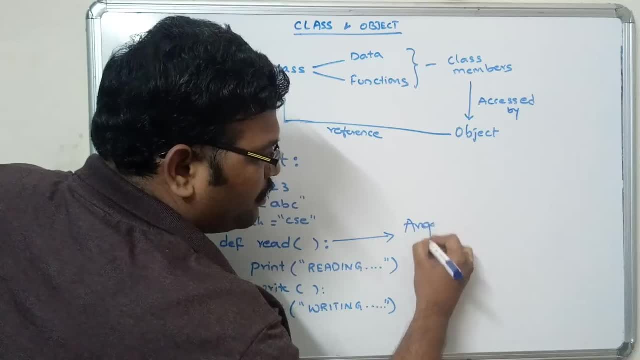 every function, the arguments lists. argument list starts with A and F means which one might be the lowest or most reasonable. argument again, adjusting arbitrary argument lists by two entries, then storm results which one might be the lowest or the most reasonable, but after class state, of course class relaxes. 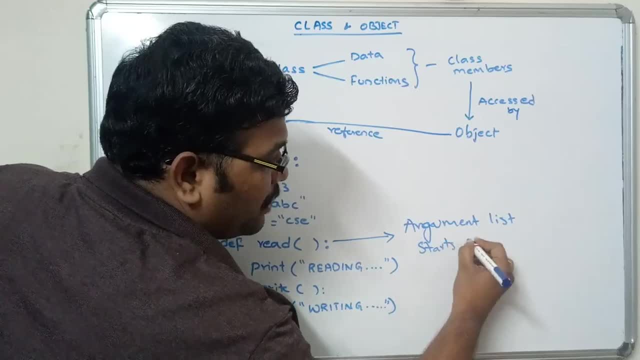 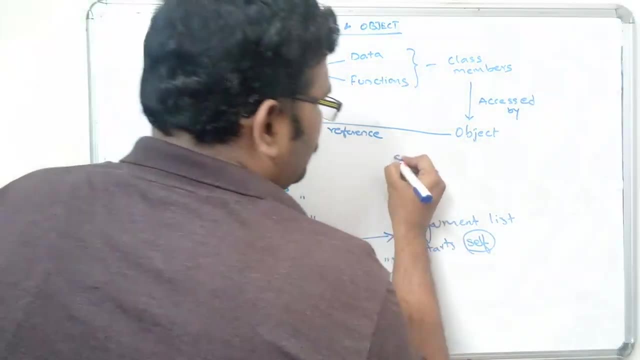 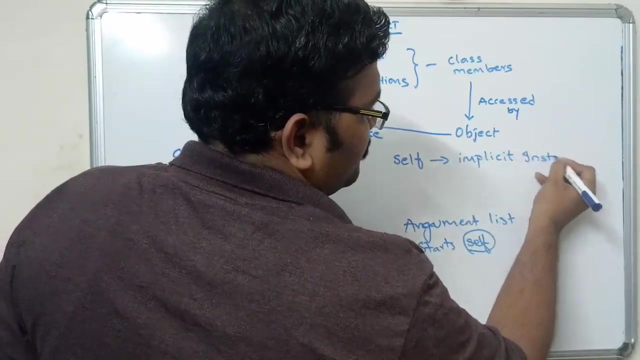 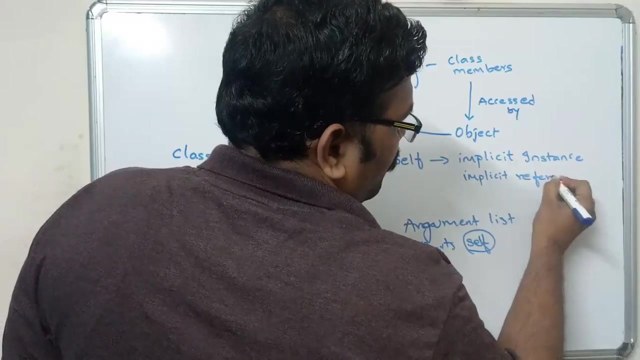 that cause Y. So bottoming down when you read a class cooker shows what a lower and lower rate Spa by problem entering a feature was your command item. OK, so with self, self, so self is an implicit instance, so self is an implicit instance or implicit reference. so if you know java, the, this keyword can be replaced with the self. 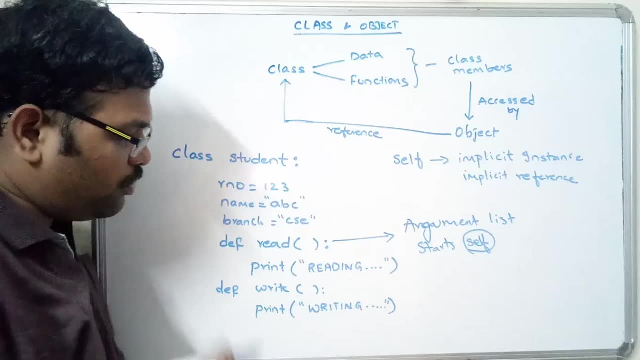 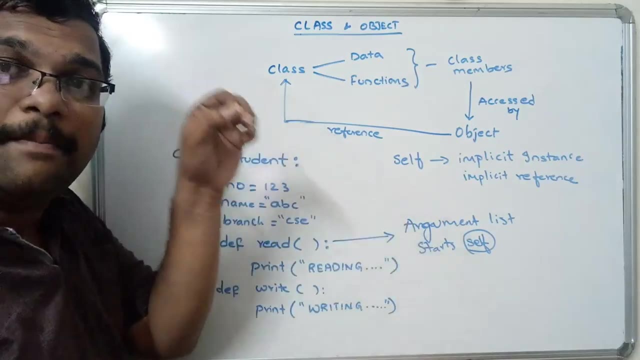 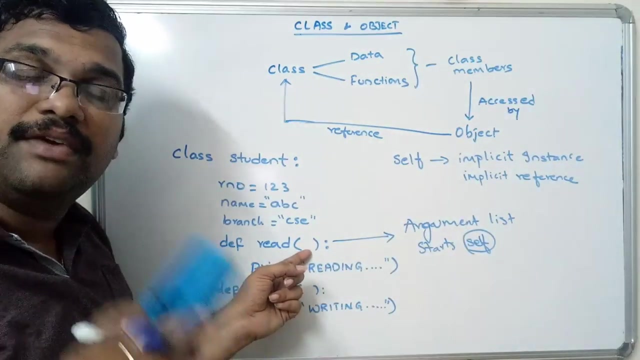 the working of this is nothing but our self. so always the user defined functions which we are writing inside the class. the argument should be self, so it is a mandatory for every function. so if you are not writing this self as a parameter to the user defined function, 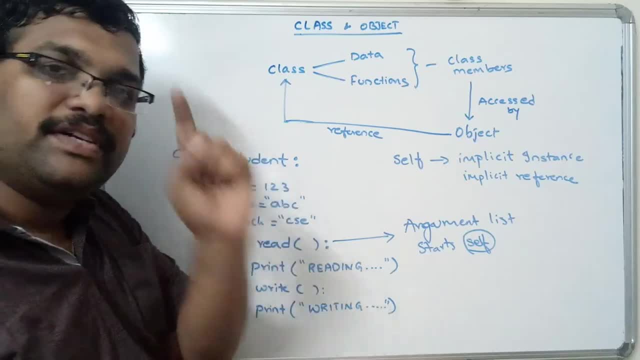 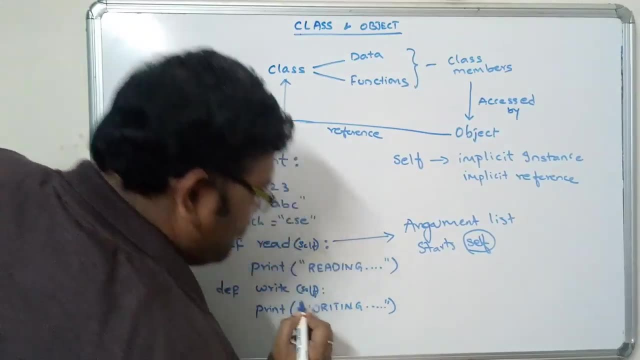 definitely you will get an error because it will treat the first argument as a self, and it is a mandatory, so here you have to write it as a set. so if, if our user defined pro doesn't have any arguments, then only one argument will be there, that is self. 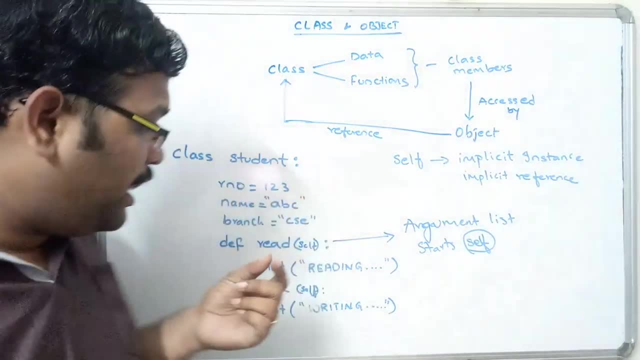 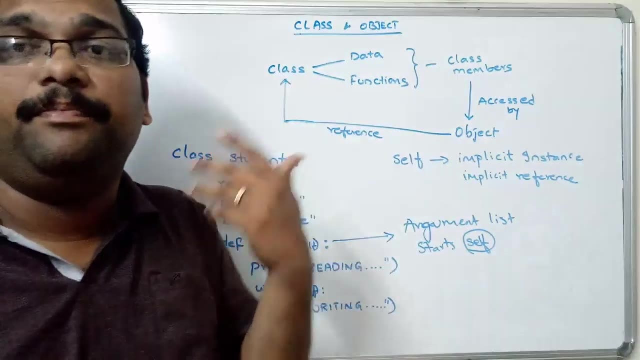 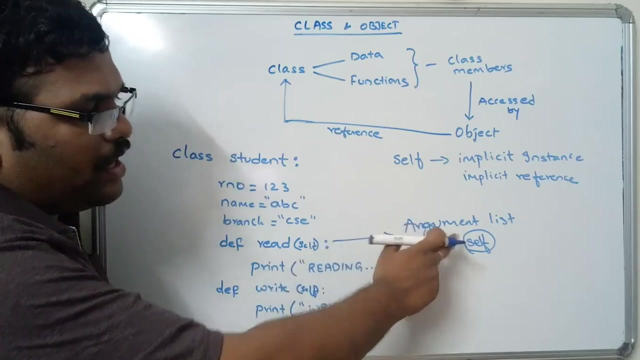 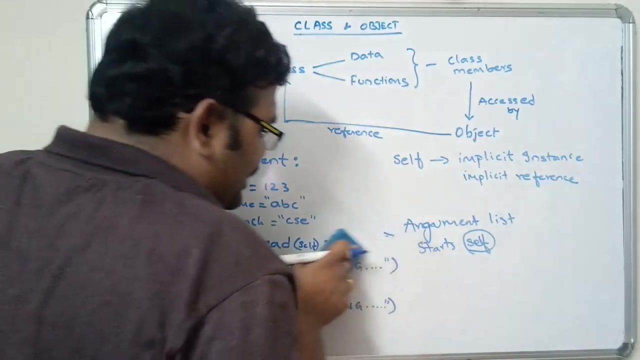 if our user defined function is having two arguments, then the first argument will be the self and the second argument will be some other variable a and the third argument will be c. right, so self is a mandatory, self is a mandatory and that is an, that that must be the first argument in the argument list. right and now. this is how we. 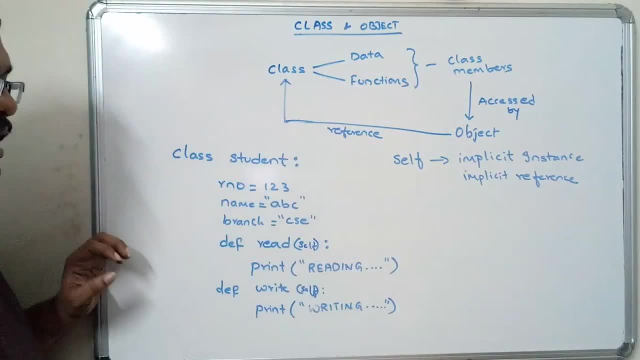 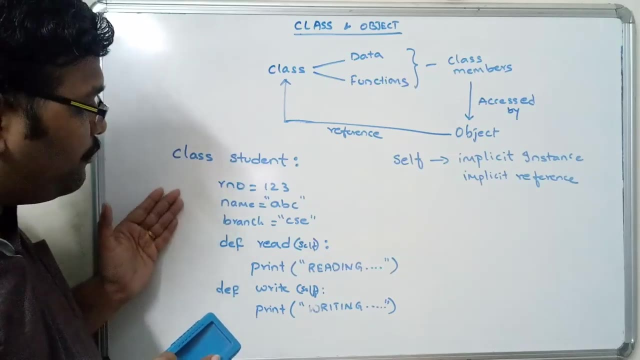 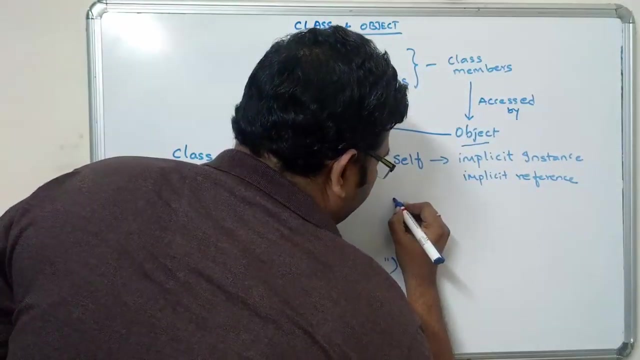 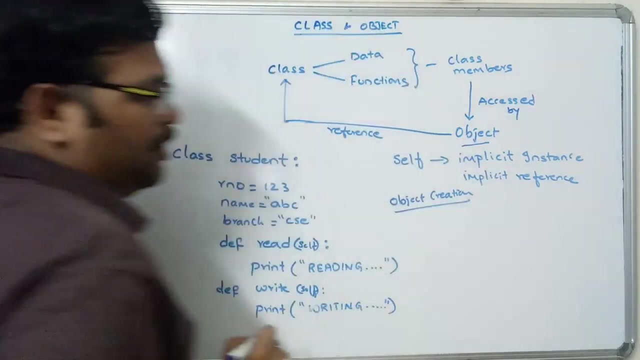 can create a class. this is how we can create a class. now the question is: how can we access these variables and these functions? and for for accessing this one, what we have to do? we have to create an object. so here the syntax for object is so: whenever you write this class, the 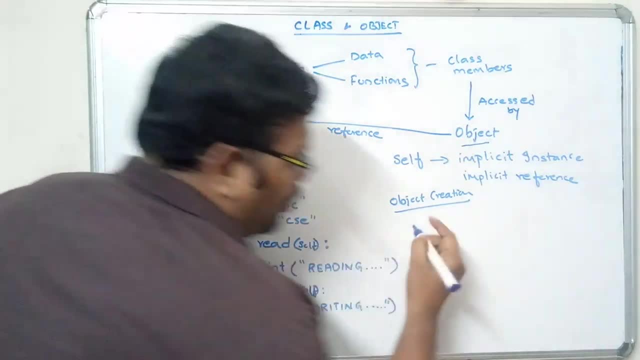 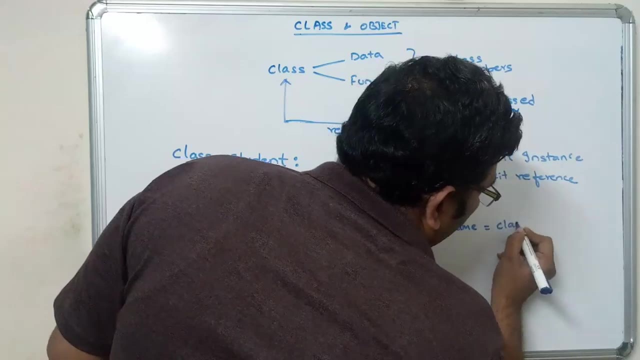 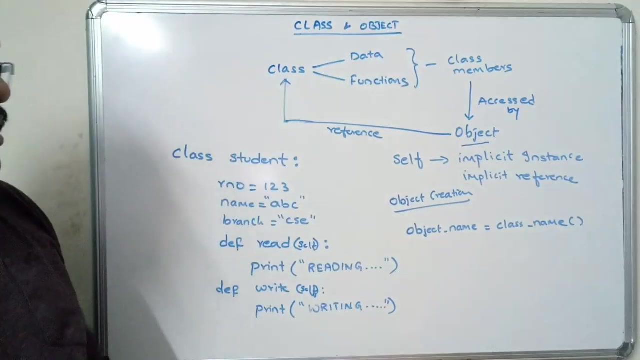 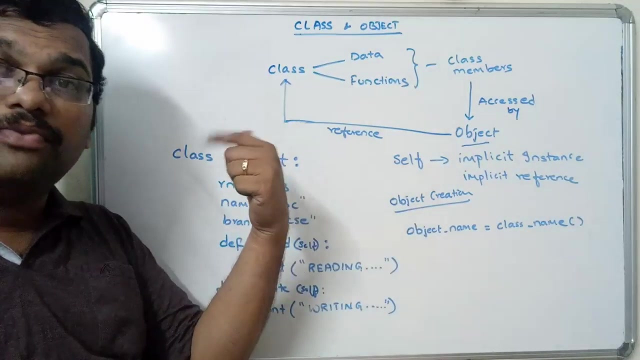 object will not be initialized until you create the object. so object is the creation. syntax is: object name is equal to class name parenthesis, class name parenthesis. so here object name is equal to class name parenthesis. here the object name is an identifier, so we have to follow the 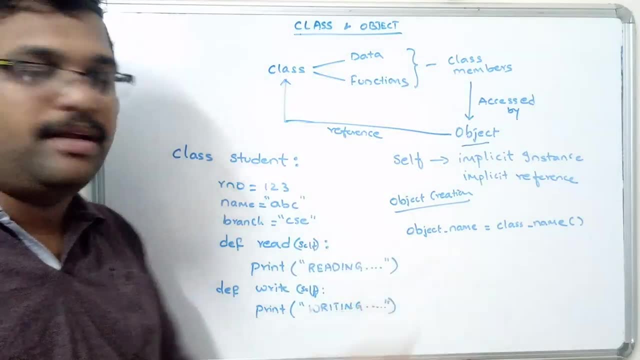 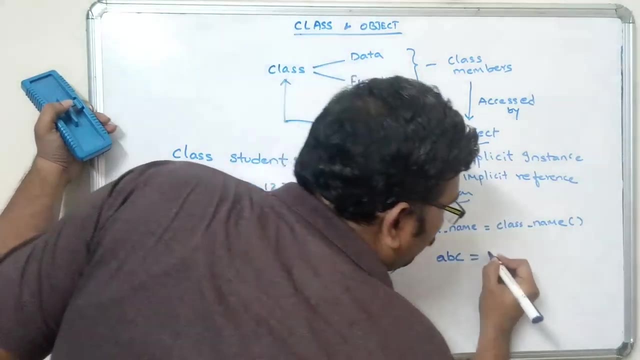 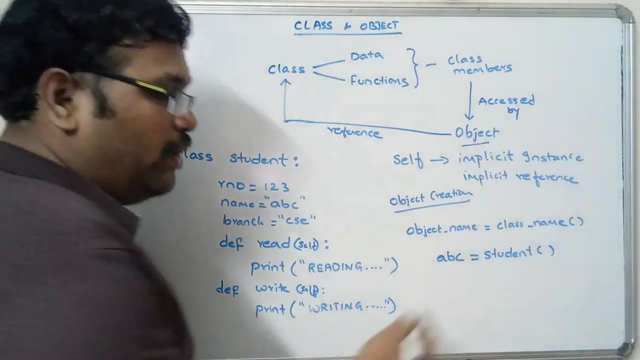 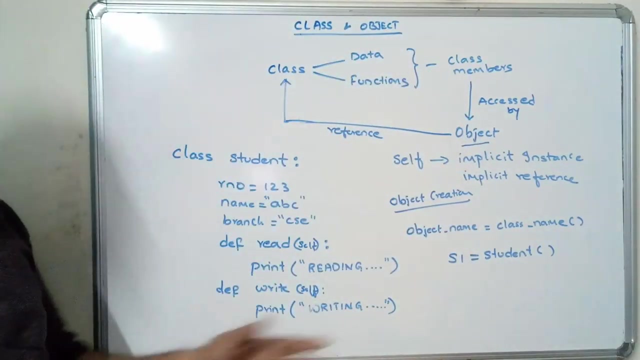 rules of an identifier before giving the name for an object. right, let it be. i am giving here some. abc is equal to student. abc is equal to student, so abc is an object, or simply we can write it as some s1. okay, s1 is equal to student, s1 is equal to student, that means the student one. so 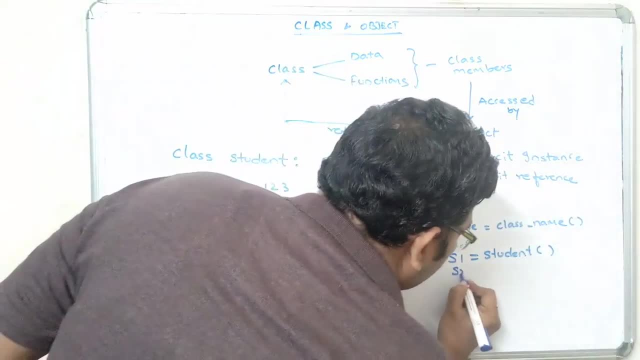 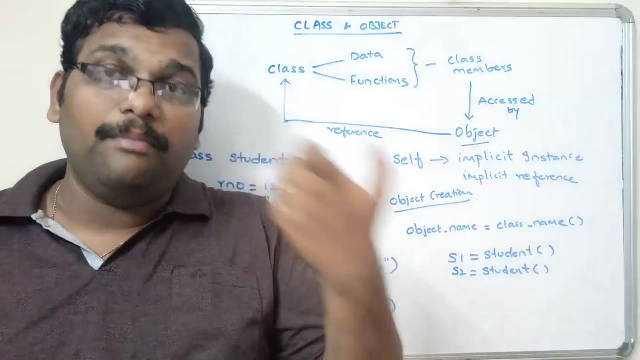 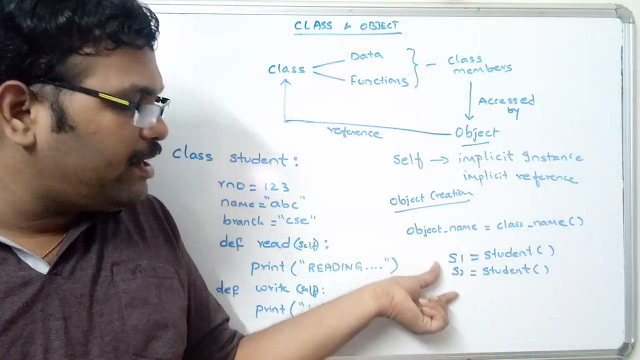 s1 is an object for student and similarly some s2 is equal to student. so we yesterday in the session i have said that one class can have multiple instances. number of instances right. so similarly one student class can have multiple objects. so here i'm creating two objects, s1 and s2. so if you want to access these data and functions of a class, simply we 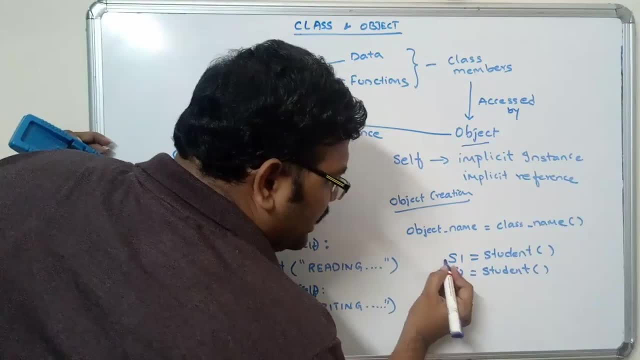 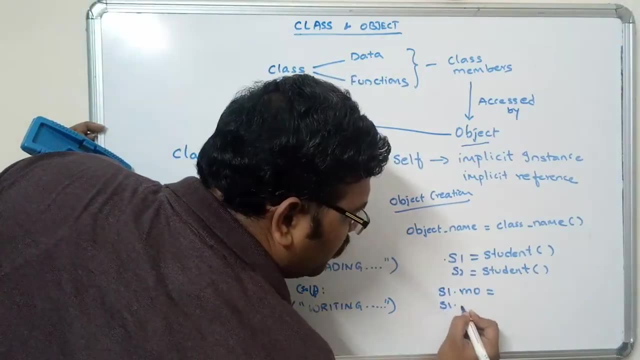 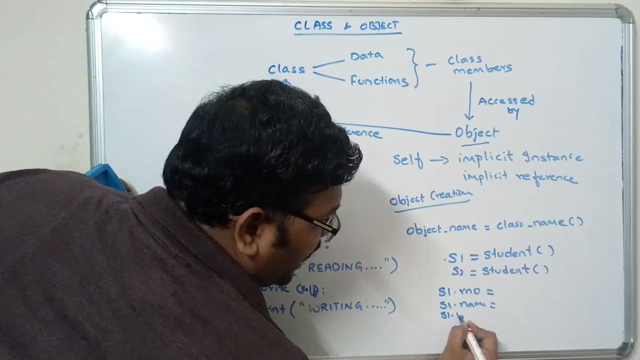 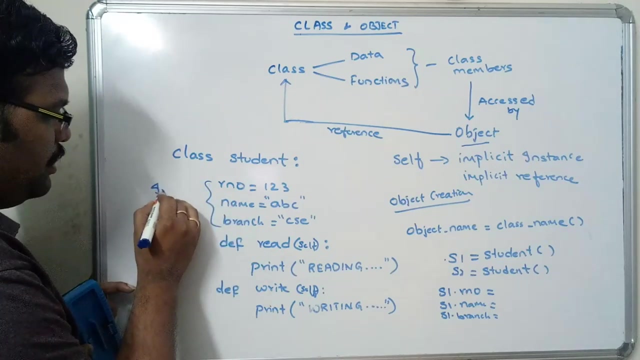 have to access with the help of the object name. so s1 dot, our number, will give the given number. similarly, s1 dot name will give the name which is given in the class. similarly, s1 dot branch will give the branch value here and these are called instance variables, instance. 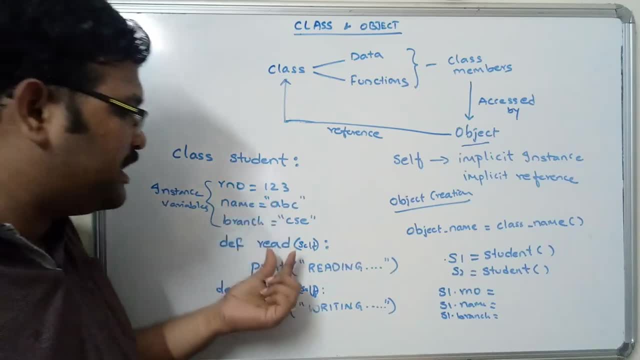 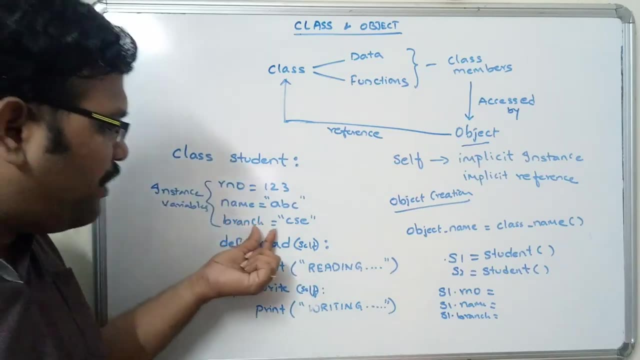 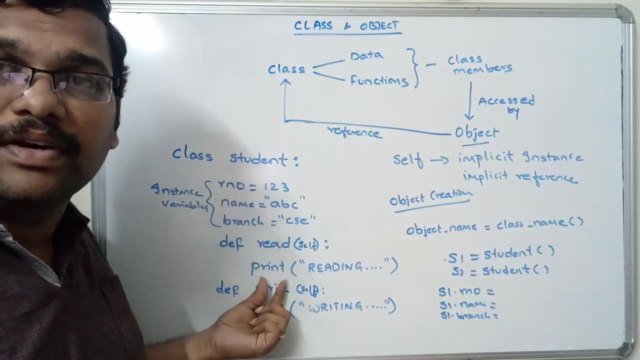 variables. so if you are creating the variables inside the function, those for those variables will be called as local variables, right? so here the variables are not a local variables. these variables are defined inside the class but not in the function. so that's the important thing you have to remember. so 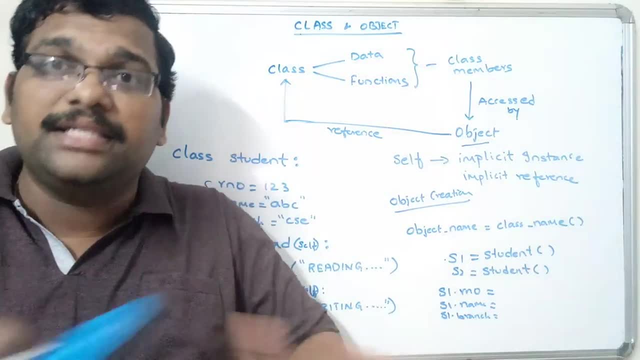 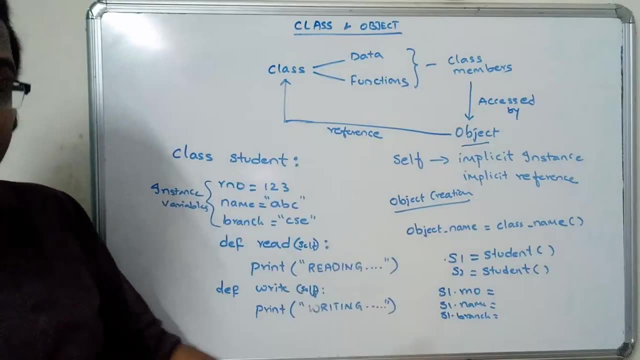 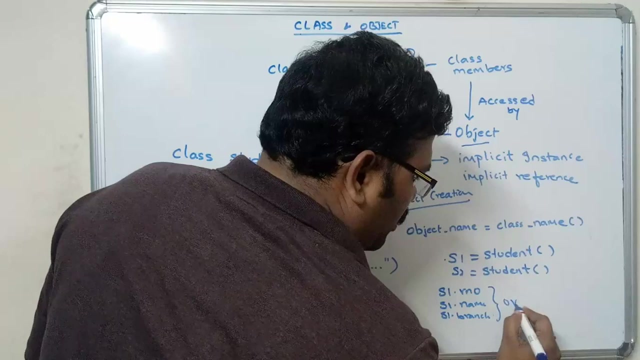 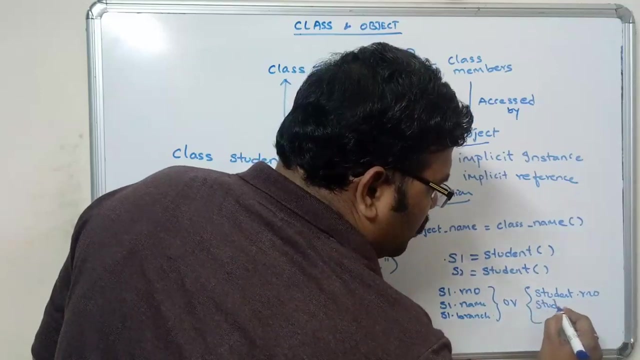 variables which are declared inside the class but not inside the function. those variables are called as instance variables and that can be accessed only with the help of object name or the class name. so we can also you or we can also access with the class name: student dot R number similarly. student dot name: similarly. 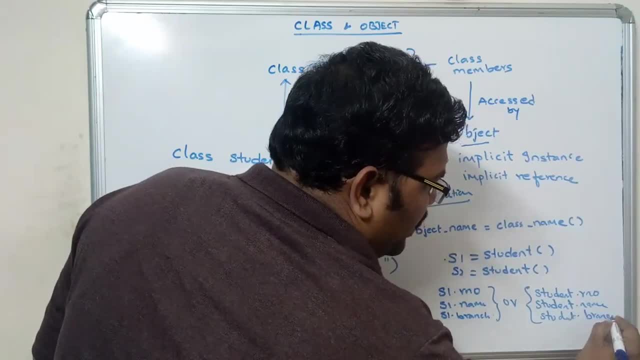 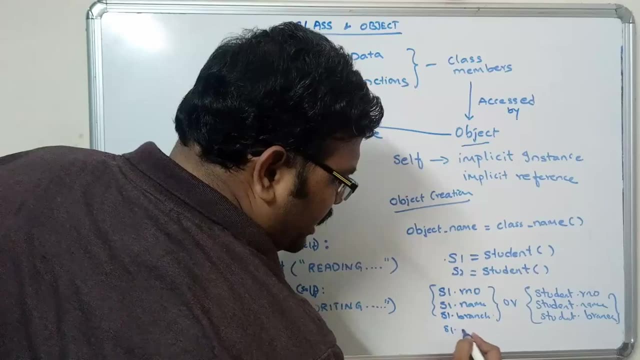 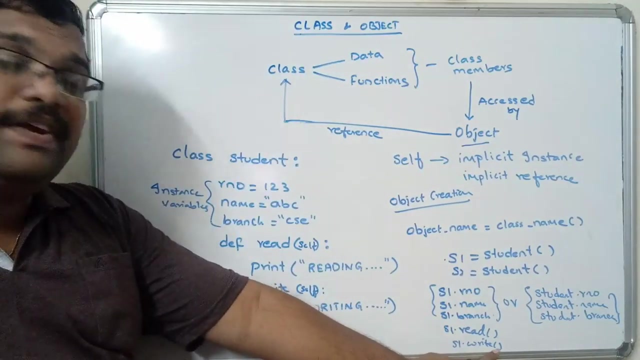 student dot branch. so in any way we can access the data. similarly, if you want to access the function, we have to write s1 dot- read, s1 dot- write. so in the function call we need not specify any parameter, but inside the function definition we have to write the self parameter and similarly. 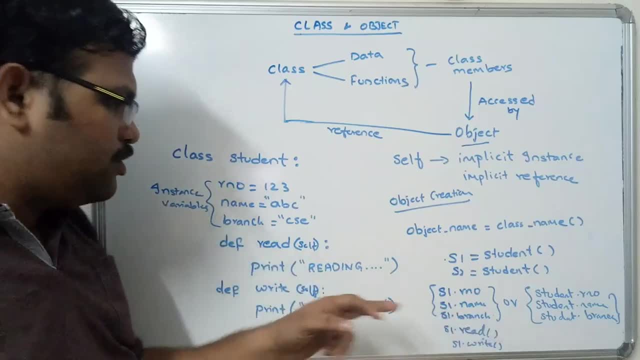 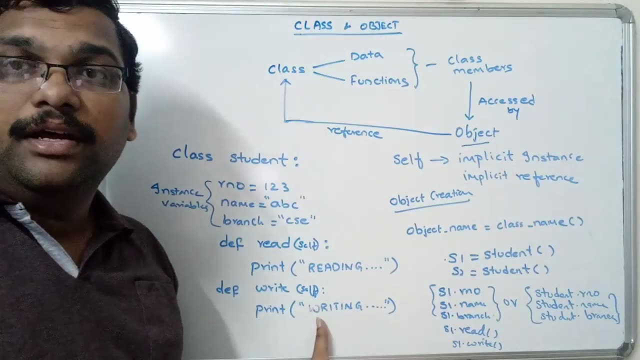 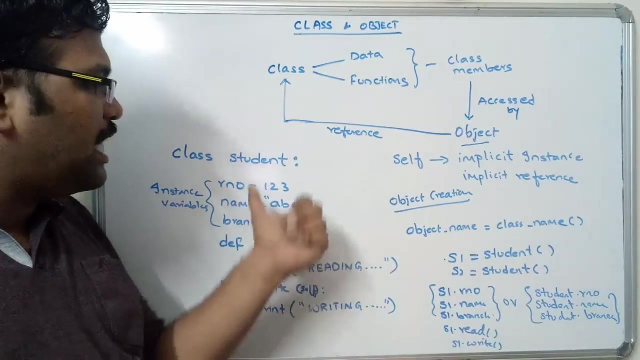 here also we can access these functions with the help of student name, so the class name, so that is a student dot read, student dot write or s1 dot read or s1 dot write. so these members can be accessed with the help of object on this class name right, and if there are local variables, that are variables which are declared. 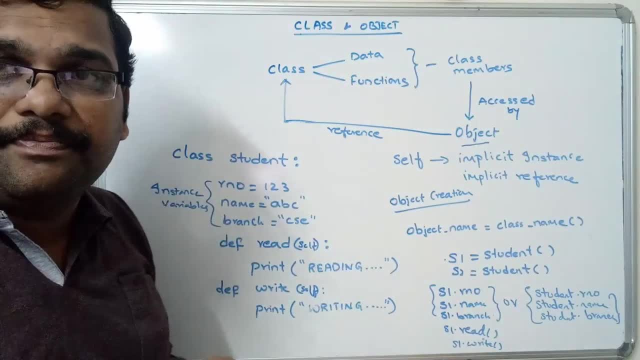 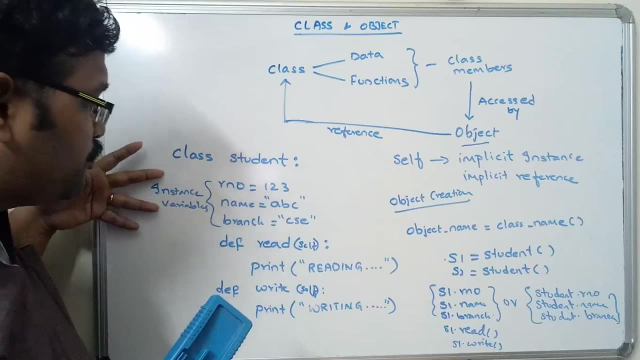 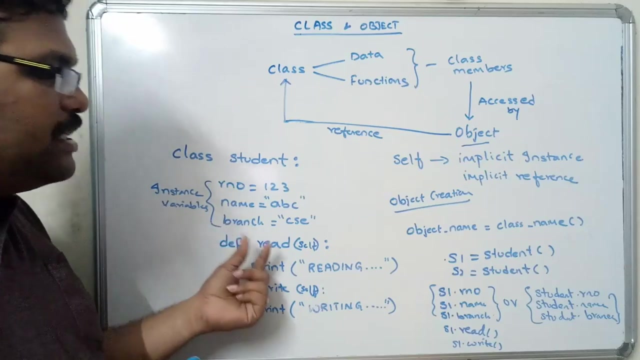 inside the function those variables can be directly accessed. okay, only the instance variables. that means the variables. so just remember: the variables which are defined inside the class outside the function are called as instance variables. these instance variables can be accessed only with the help of object name or a class name. so this is all about. 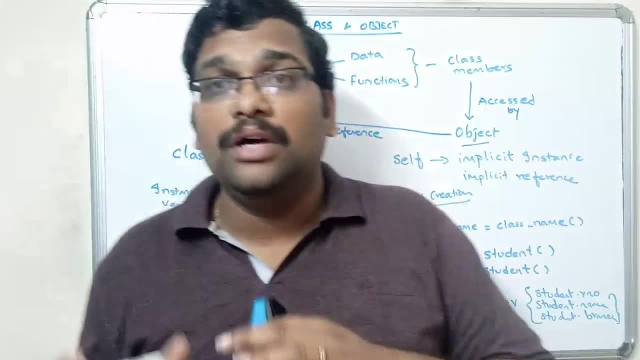 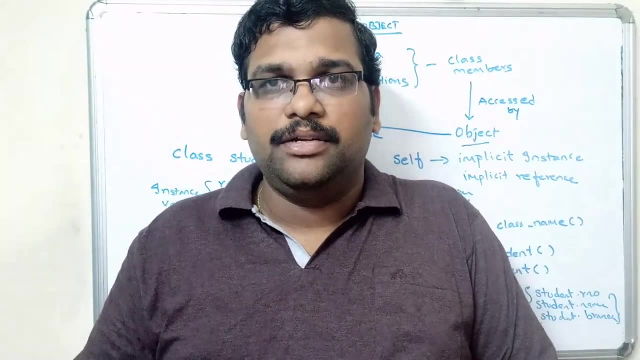 our class and object. so how to create a class and how to create an object. so a class can have a data and a function. both we call it as a class members, so in order to access those members we have to create an object. so object creation syntax is this: one object name is equal to. 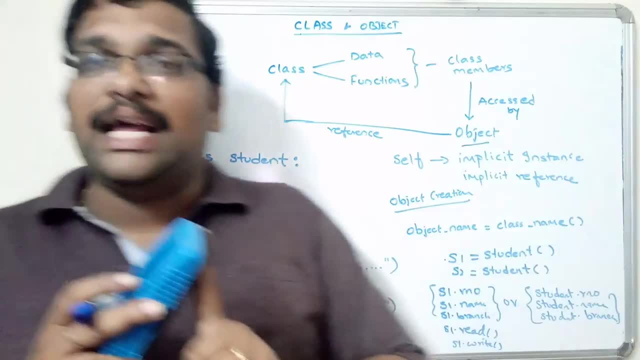 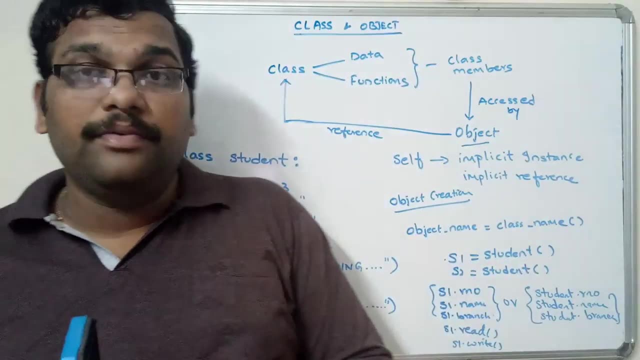 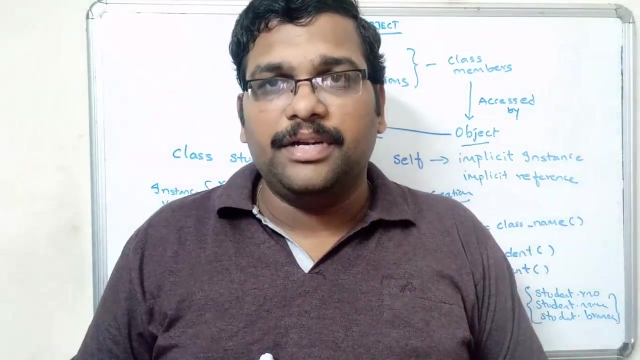 class name parentheses, so one class can have multiple instances, right. so we'll stop here and we'll see the implementation. so how to create an object and how to create a class and how to access the data members. i mean class members, that is, a data and functions. so we'll move on to the interpreter. 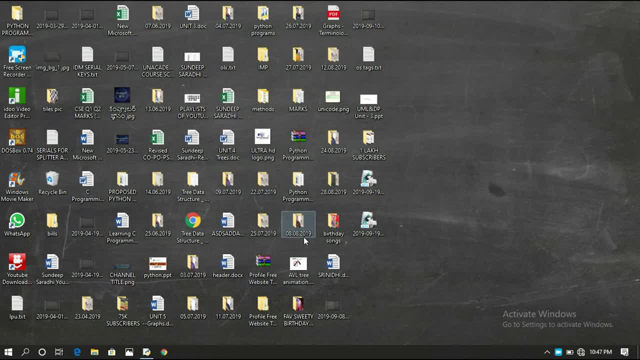 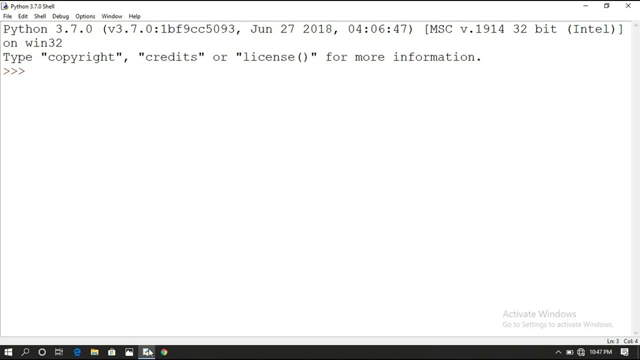 hi friends. so just now we have seen how to create a class and how to create an object for that class and how to create a variables and the functions. so we we have said that a class can have a data and a functions. right, so how to create that one? let us see this one now. 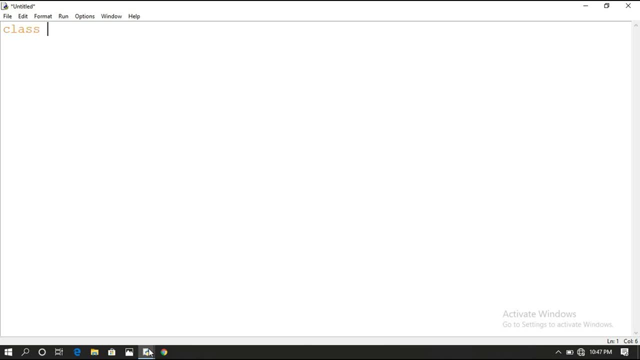 so we have to begin a class with the class keyword, so class, followed by the class name. so let us take student as a class name. so a class is a block of statement, so, which contains the variables and functions, so student. so here we can give a student variables, different variables, so let us take some. 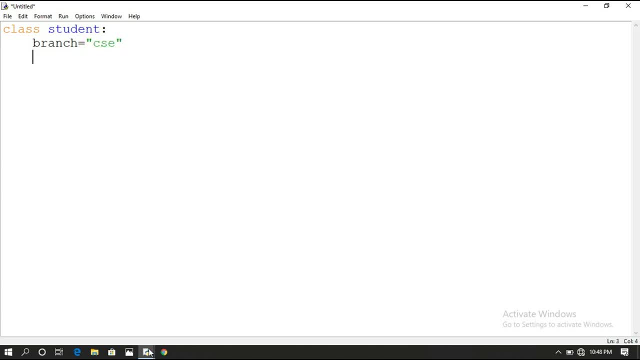 some branch is equal to csc and i am writing the function def. so in python, every function use a defined function should start with the def keyword, so df, so read. so i am writing some READ. so we have type酵 used to define a function should start with the def keyword, so red, so read. so i am writing a reason as to why it is called DEF key words which i am editing this video. 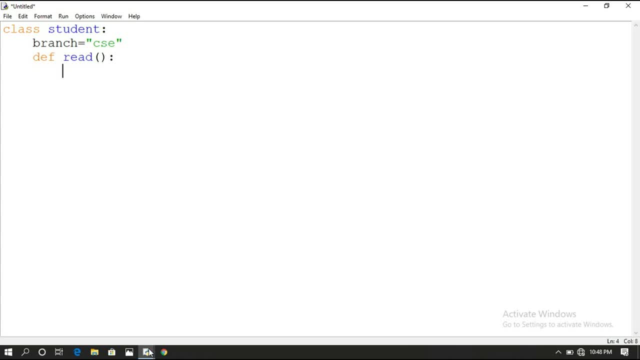 So I am writing the read function So a student can read: ok, Student will be having some branch role, number, name and so on. So R number is equal to 1,, 2,, 3 and similarly, name is equal to some ABC right. 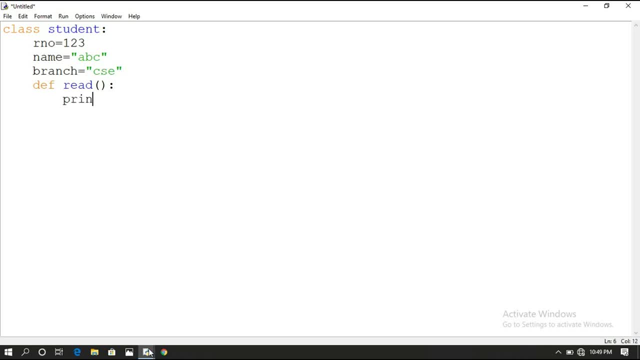 So read function, So read. just. I will write a simple thing. Print reading right, So let us close this. So this is a class, So which can have the variables as well as functions, So we can write a multiple functions here. So a class can have a multiple functions and a multiple variables. 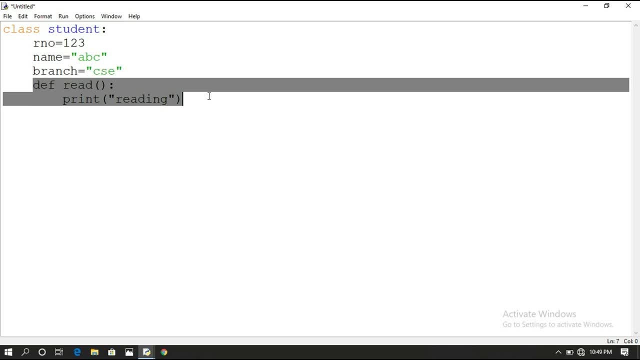 Now, in order to access the function of this class, we need an object. So without creating an object, we cannot access these variables or these functions inside the main function. So here I am: creating an object, So ABC is equal to. So this is the syntax for creating a object, So ABC is equal to student. 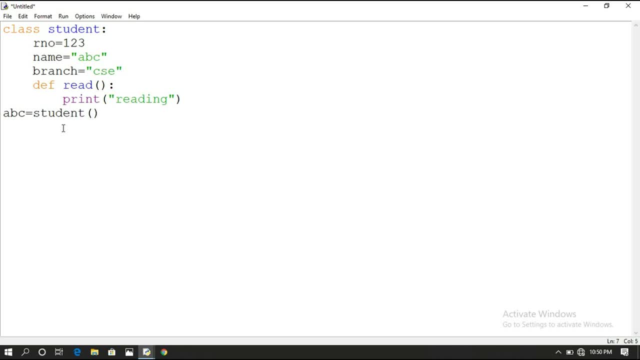 Now ABC is. It is an object for the class student. So in order to access the objects or variables of a student, that should be accessed with the help of object name. So print ABC R number is equal to object name, dot R number. So without using the object name it cannot be printed, right. 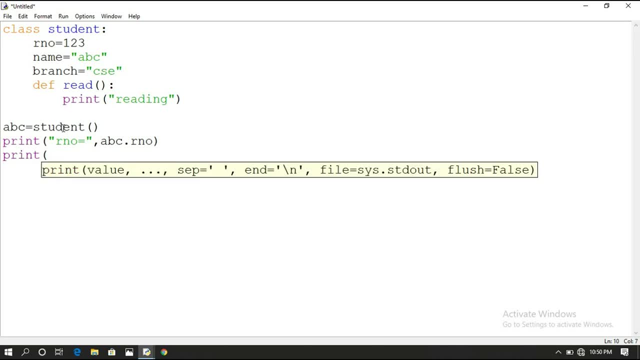 Similarly, print Name is equal to name, print branch is equal to branch right, And if you want to access the function, that also should be done with the help of ABC, ABC dot. Sorry, here I did not access These members using the object. 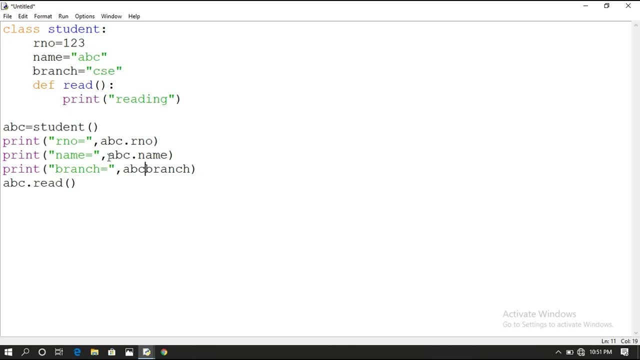 So once again, I'm repeating: So if you want to access the class members, and that should be done with the help of the object created for particular class, So here ABC is an object created for the student class. So in order to access the variables and functions available in that student class, that should be done with the help of this object, ABC. 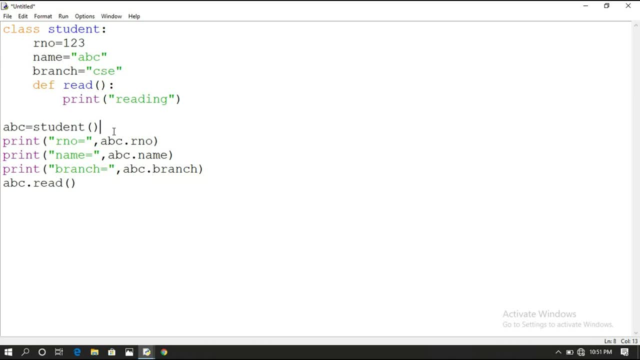 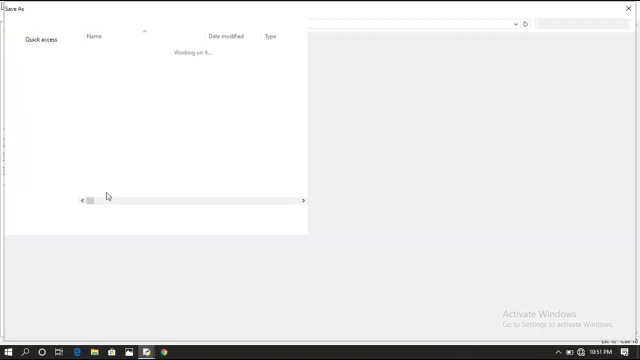 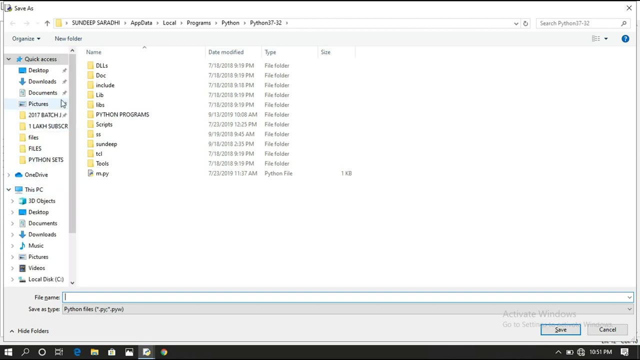 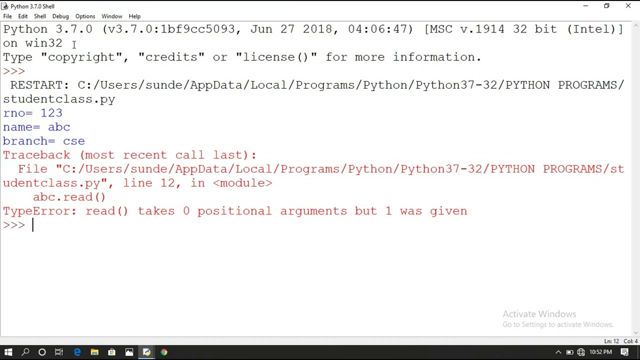 And a class can have a Multiple objects, right, So I will just save this one. So here I am saving that one. So student class dot py. Okay, I will run this one So you can get this R number, ABC and the branch. 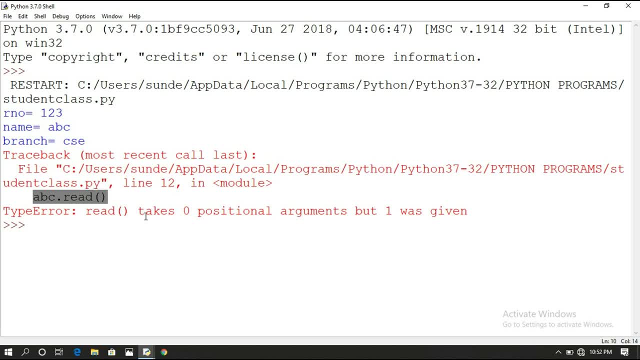 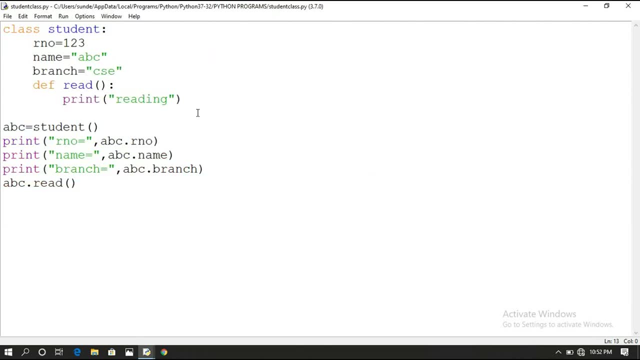 And here you can observe that ABC dot read is having an error. that read function takes a zero positional arguments, but one was given. So why? Because here, if you are writing any function or if you are defining any function inside the class, 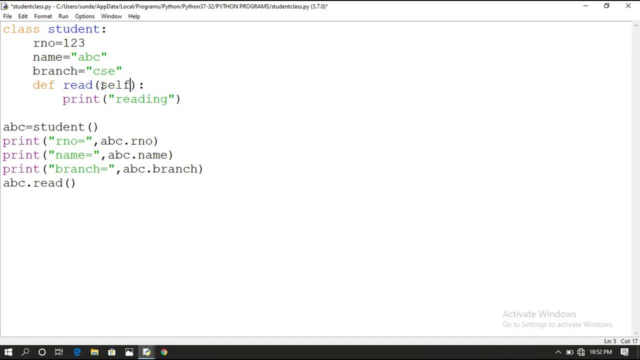 One argument is compulsory, that is, a self. self is the first in the argument list. self represents the reference or the instance of the same class. instance of same class. So we have to pass self as an argument for the function which we are writing in the class itself. right? 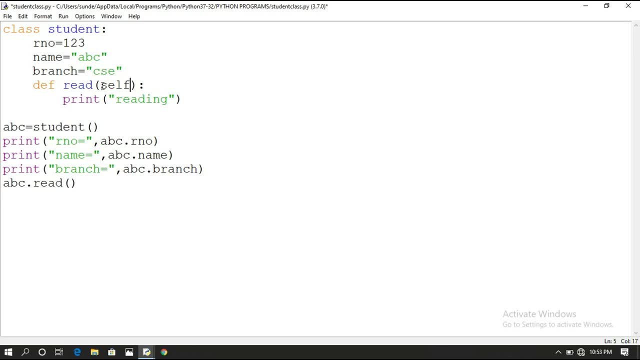 So the parameter list will start with the self. So if you are writing two parameters First, We have to start with the self. self, comma A, comma B, right. So self is a mandatory. Now you can observe if you run this one. 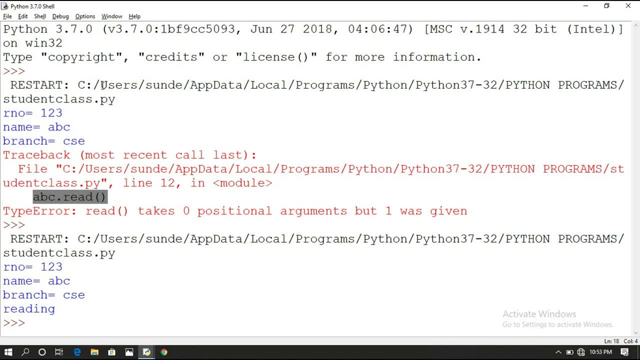 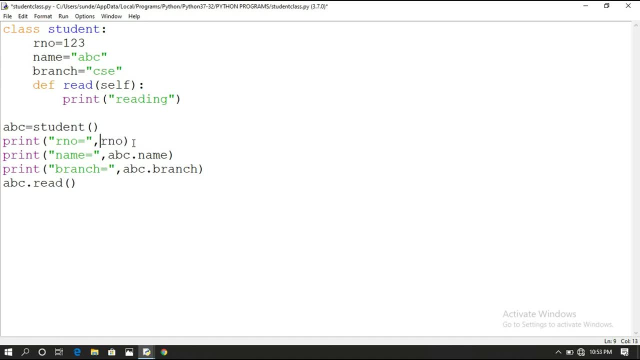 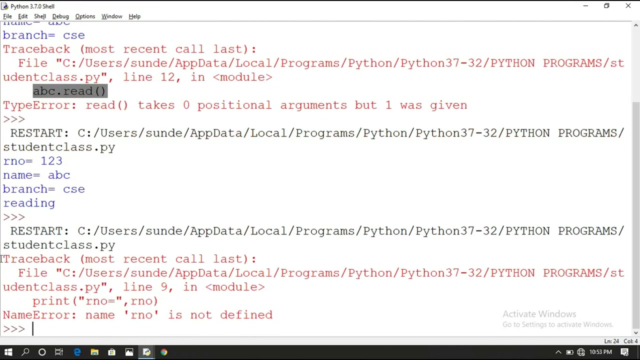 So you will get the result that the R number, name, branch and reading: So if you are trying to access without the class name, what happens? So what happens? So what happens? see, you will get the error right because name r number is not defined, so here r number is. 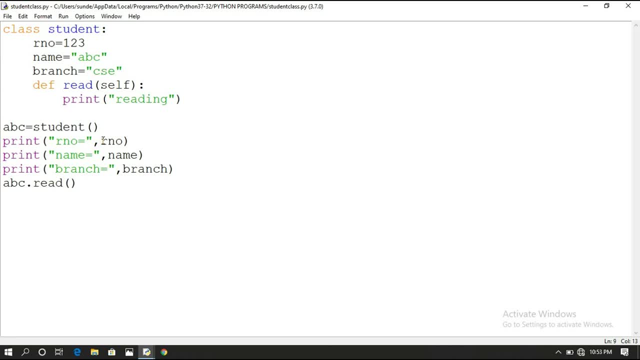 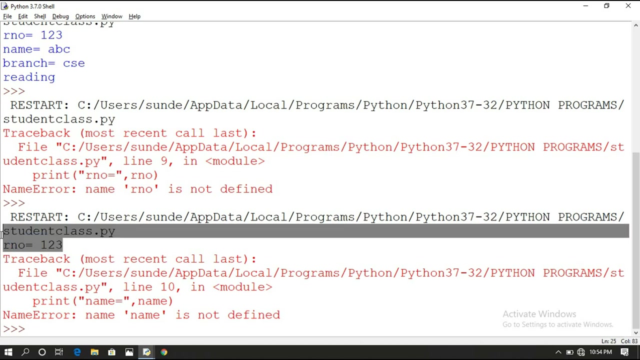 not defined because r number is the variable declared inside the class, so it's an instance variable or a class variable. so every class variable or an instance variable can be accessed only with the help of the object name or a class name. so you can observe: see, r number is equal to 123, so a, an instance variables can be accessed through the object. 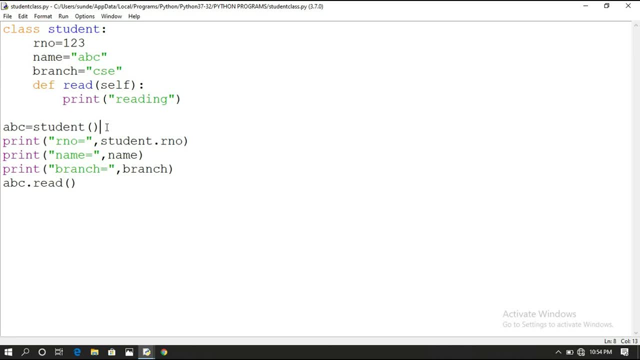 name or a class name. so once we have to create an object and then we have to access with the object name or a class name, right, right, and now see, see, and now see if we are having the same thing: three, four, five, and here, if you are trying to print r number c, so already we know that. 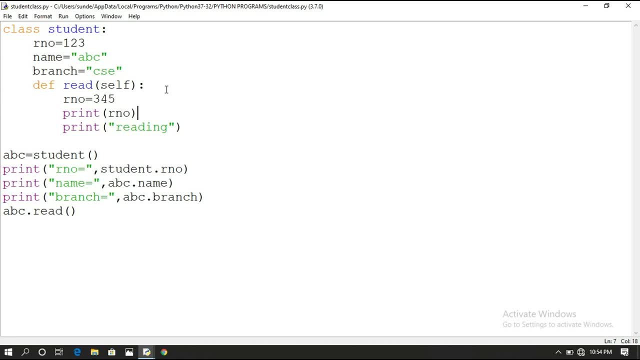 uh, the user defined function may also have the variables right, not only the class. user defined function may also have the variables. so these variables which are declared inside the class and outside the function, those variables, we call it as class variables or instance variable. so these variables should be accessed only with the help of 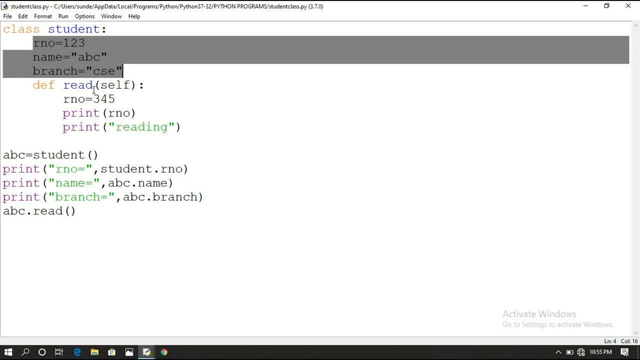 function, i mean class name or object name and whatever the variables we are declaring inside the function of a class, those are called a local variables, so they can be directly used in that function itself. so if you here see, observed so, so i'm taking a different name. so role number is: 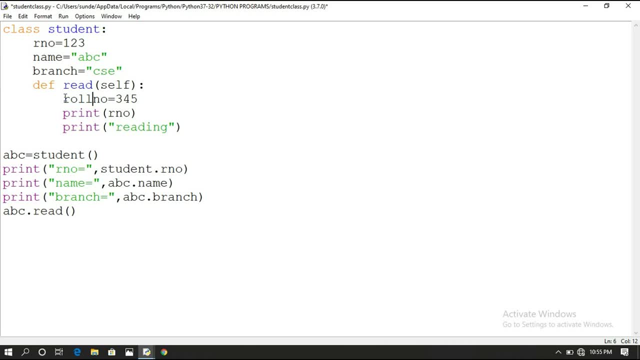 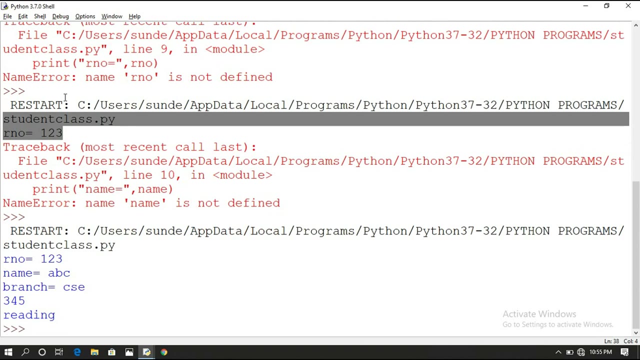 equal to 345. that is a function name. so i'm taking a different name. so role number is equal to 345. that is a variable declared, initialized inside the function. so i'm printing the same thing, role number, so you can observe here. so even though we are executing, so we can get that r number is equal to 1 to. 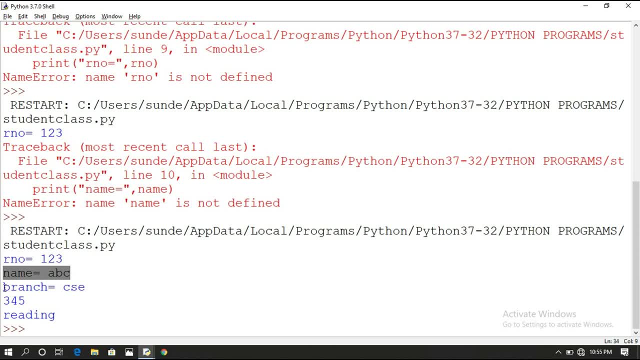 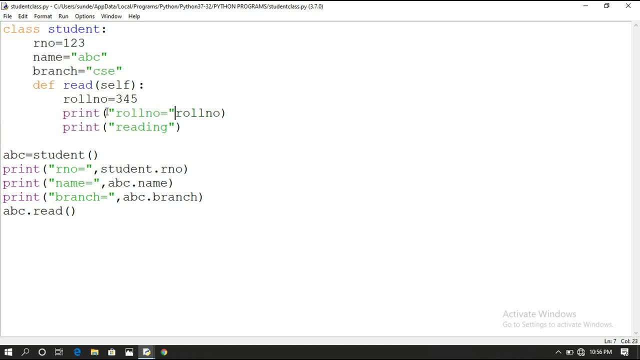 23. name is equal to abc, branch is equal to cac and 345. here we are getting right. so, so, so, so, so it's very running long. we are. we are trying to explain the same thing right now. if so, these are the instance variables and this is the local variable. 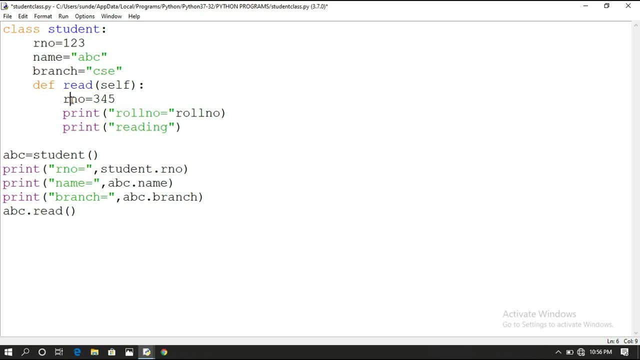 right now, if the local variable and the instance variables are sharing the same name, the first preference will be given to the function, see so here only the r number. so whatever the variable, we are sorry, right, right, right variable- we are declaring inside the function that will be displayed here So you can observe. 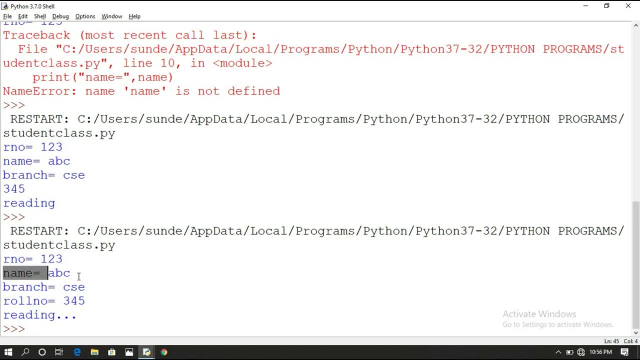 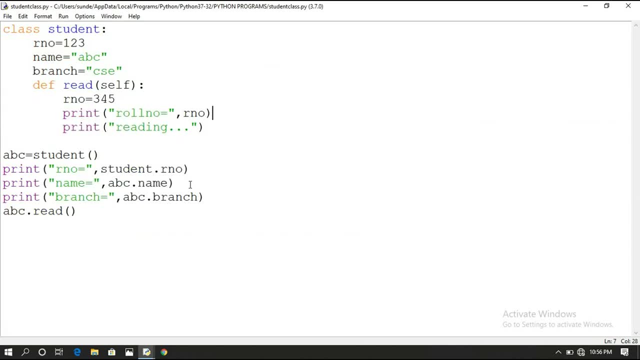 here. So r number is equal to 123, name is equal to abc, branch is equal to crc and roll number is equal to 345.. This is the thing we have written inside the main function, inside the read function, and if you want to access the instance variable inside the function, then that can be done with. 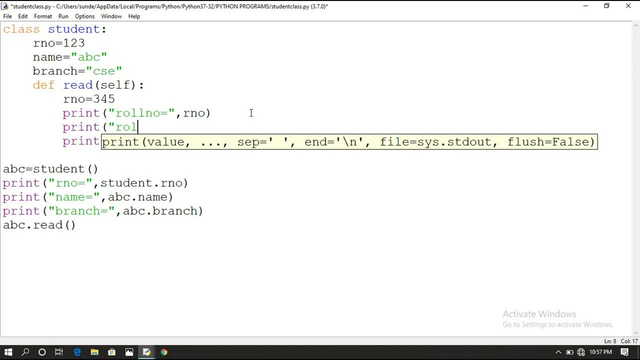 the help of self. So r number is equal to self. sorry, here I will write here: instance variable is equal to self, dot r number. So self is nothing but the implicit reference, implicit reference or implicit instance. So without creating an, 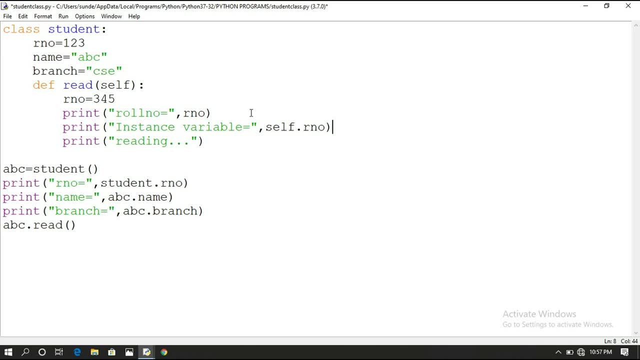 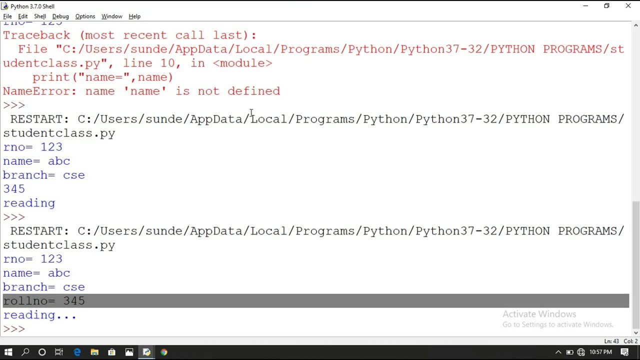 object. we can use the instance variable. So we can use the instance variable to create an object. We can use the instance variable with the help of self. So self dot r number. So this will give the instance variable. See here you can observe that. See: roll number is equal to 123, name is: 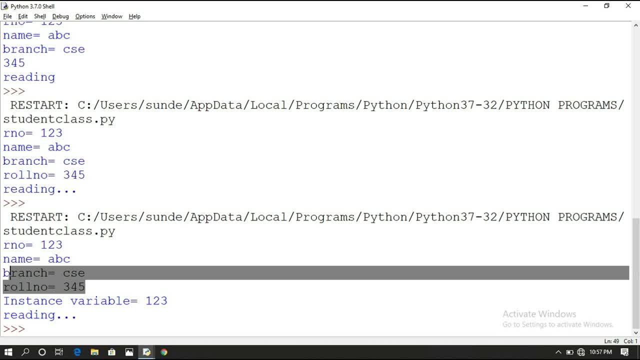 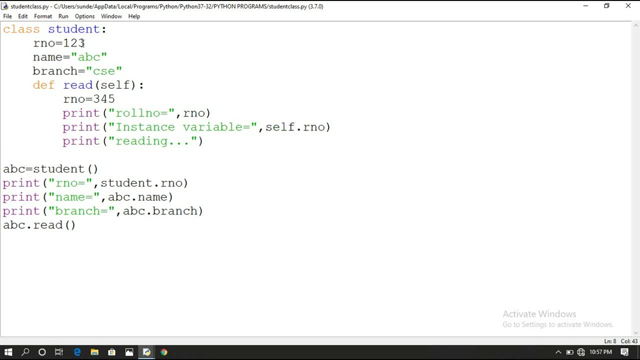 equal to abc, branch is equal to crc. here roll number is 345 and instance variable is 123, because here we are giving self dot roll number, which is nothing but 123, self dot Self is an implicit instance variable. implicit instance variable, So we can use the instance variable. 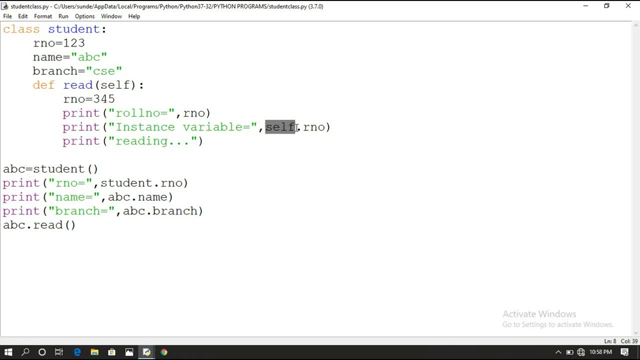 of a class. So all the variables which we are declared inside the class can be used with the help of self inside the function And outside the function, outside the class. if you want to access the variables and functions, that should be done with the help of the object. So a class can have.